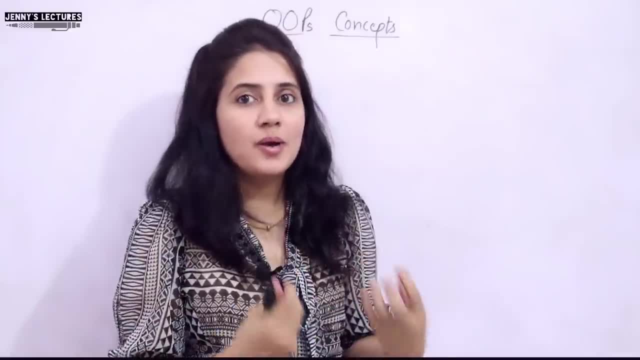 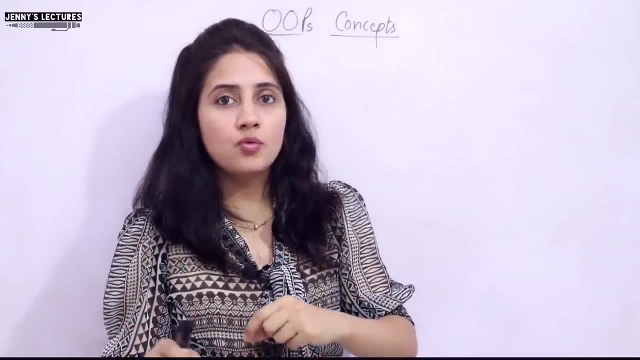 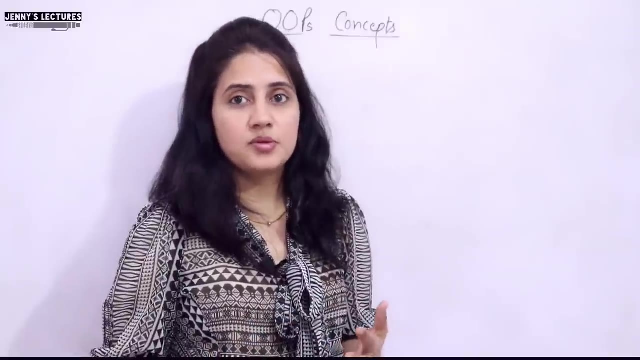 the object-oriented programming in C++. you must have some idea about the concepts, The you know the things. Because of those things we call it as object-oriented programming. What are those concepts? Like class objects, abstraction, encapsulation, inheritance, polymorphism. 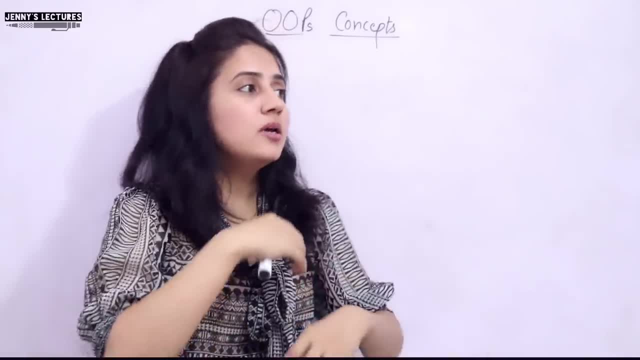 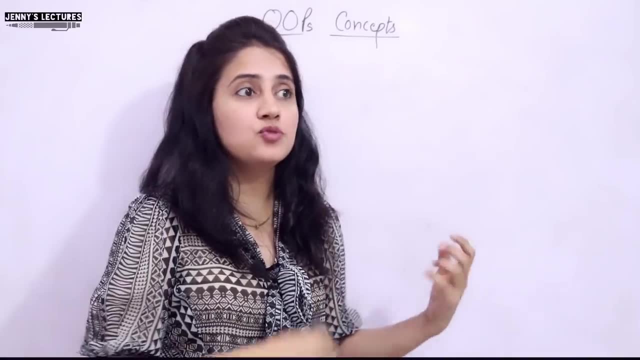 Six concepts are there. So in this video I am going to talk about these concepts briefly. I just want you to get familiar with these concepts In detail. we will discuss about these concepts one by one in later videos, Once we will move, you know, deep down into C++ course, right, But at 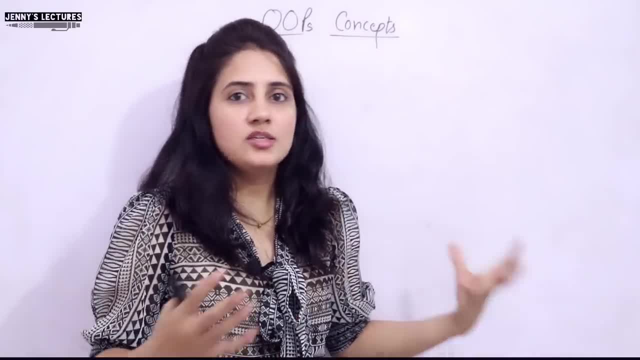 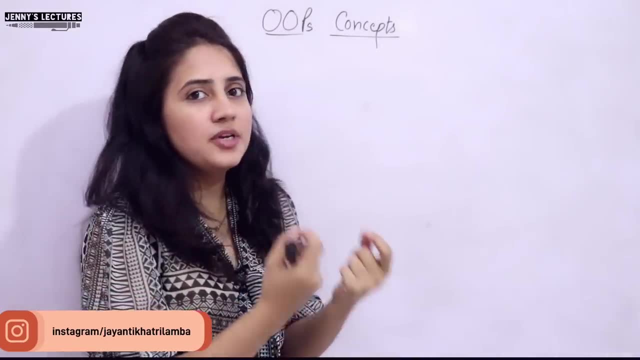 first, you must be familiar about the concepts. So in this video I am going to talk about the concepts Like: what are these concepts? At least the basic idea you should have, right? So those things we will discuss in this video, Every concept in brief. I will relate it with the real. 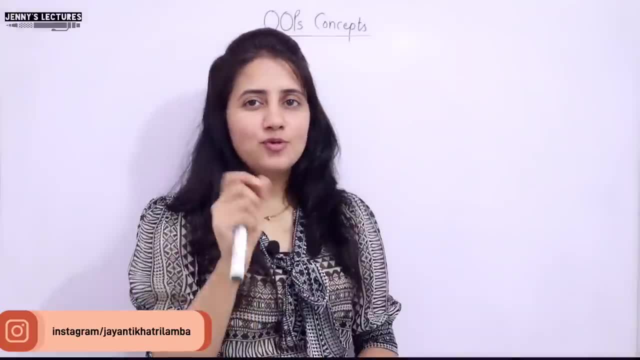 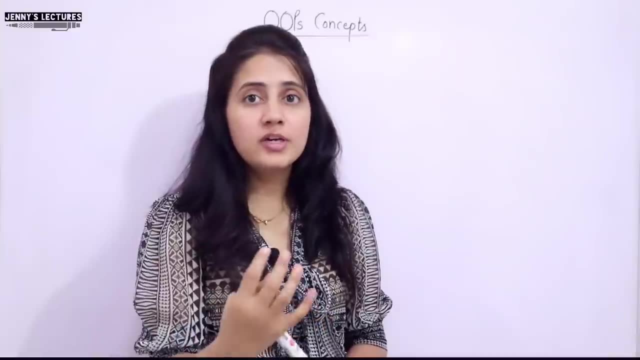 life example. I hope you will get it right, But before that I just want to tell you one thing: With theory, practice is also important. The key to success in any interview, specifically in programming interview, coding interview- is practice, Practice as much as possible. It's. 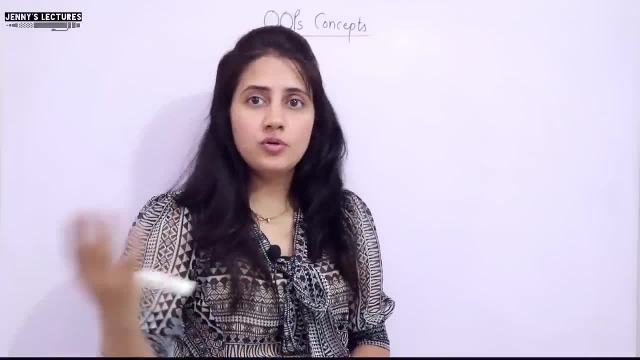 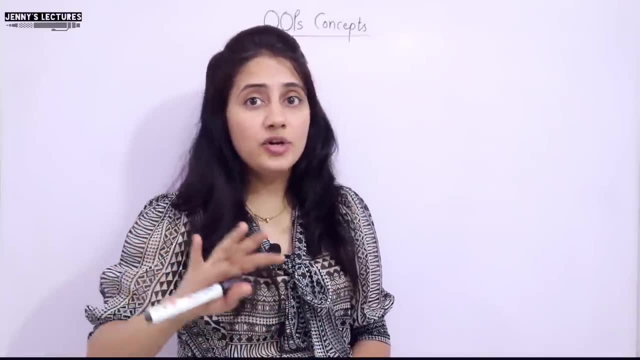 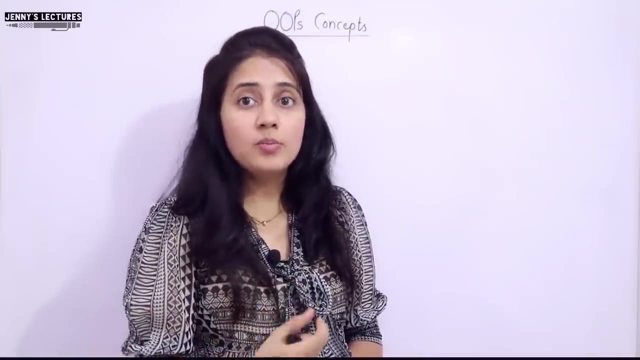 not, like that, start practicing coding problems, just you know, few days before your interview. No, The best method of preparation is incorporating your interview preparation into your everyday coding practice. It will help to improve your logic building skills, your thinking capability, your problem solving skills. and that's exactly. the industry wants a problem solver, But the 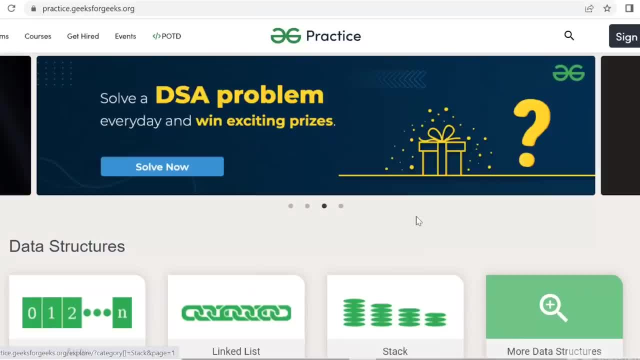 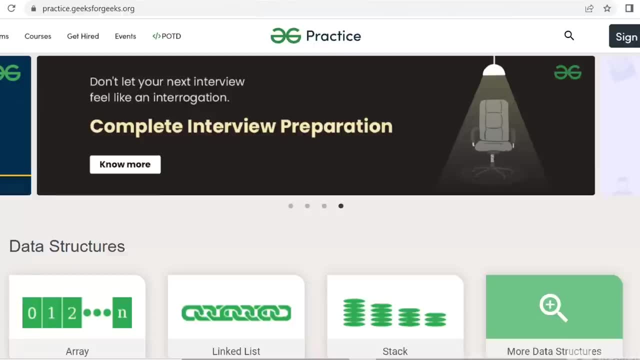 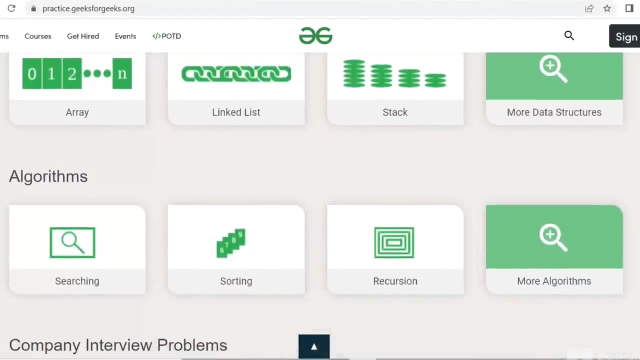 question is how to get started from where you can practice the problems, coding problems. So here is the solution. This is the practice page of Geeks for Geeks. Here you will get many coding questions, Different topics like from DSA Array, linked list, stack In algorithm. 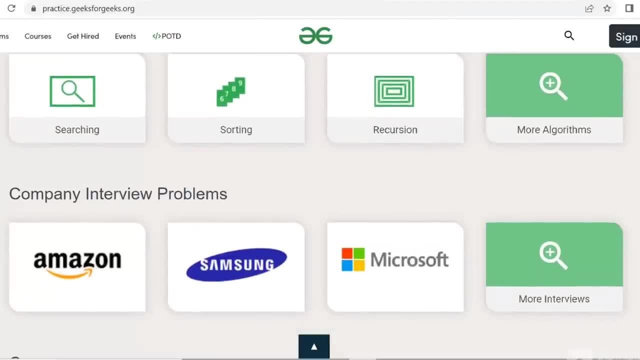 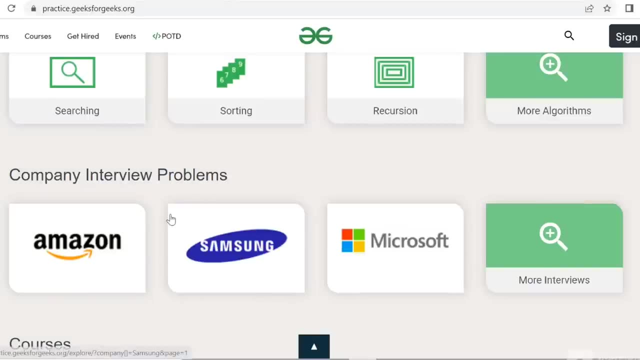 you will get different coding questions on the topic searching, sorting and many algorithms based on many algorithms, As well as company specific coding questions. Practice questions you will also get Suppose if you want to practice the problems which are being asked. 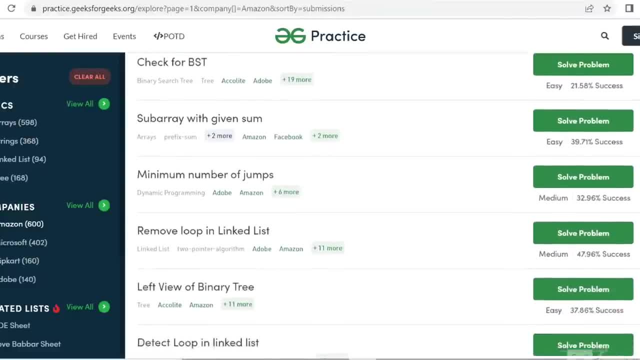 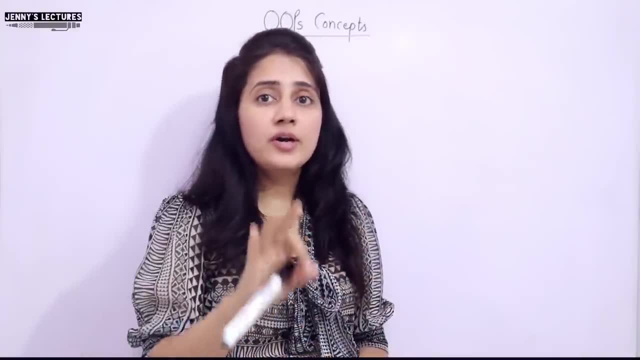 in Amazon interview, then just click on that and you will find out the list of problems and you can start solving these problems. and it is not just just the problem solving, that is a problem solution good for students only, but as well as for working professional. if you are working somewhere and you 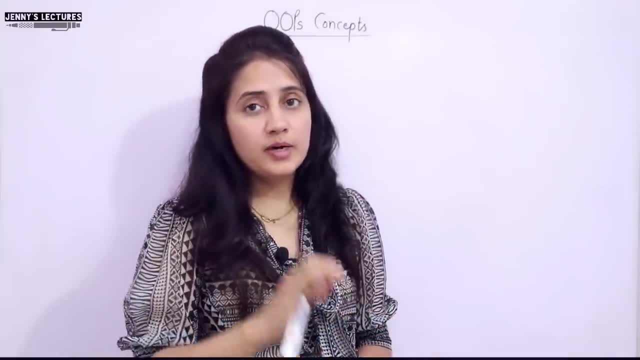 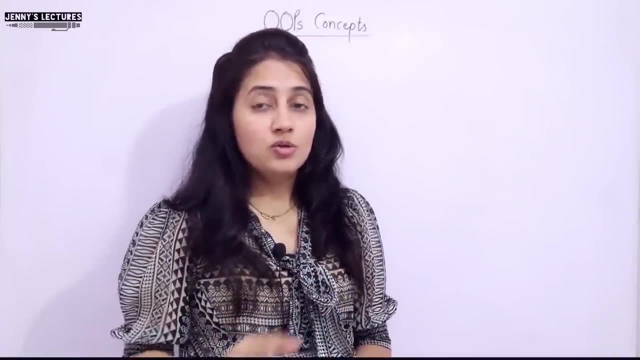 want to switch or applying for new position, then also it will help you. practicing these problems will definitely help you. so i think this is a great resource to practice these coding problems. don't worry, the link i'll put in the description box of this video. you can go and. 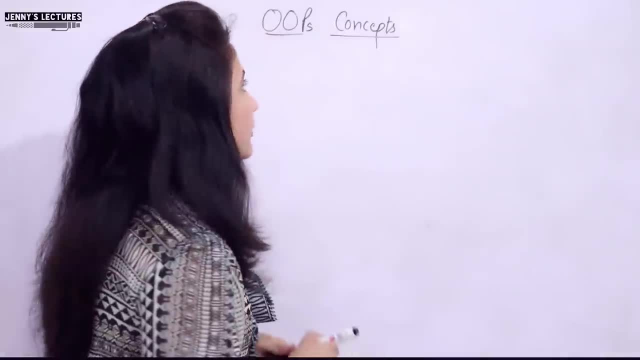 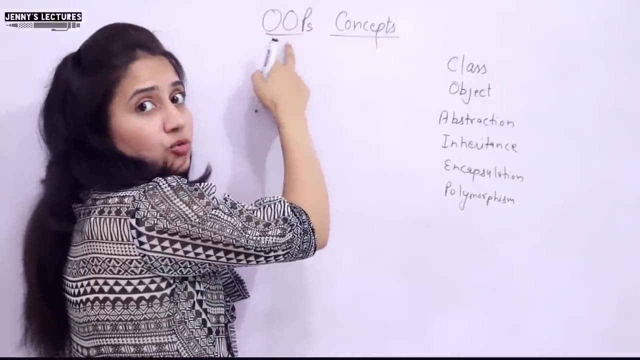 check out. now let's back to the topic. so what are oops concepts? six concepts are there. basically, these are six concepts. in object oriented program, see, as the name suggests, object oriented. so obviously object is the main thing. everything revolve about the around the object, so you'll. 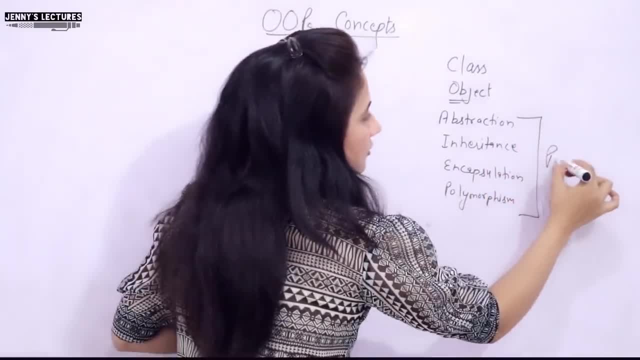 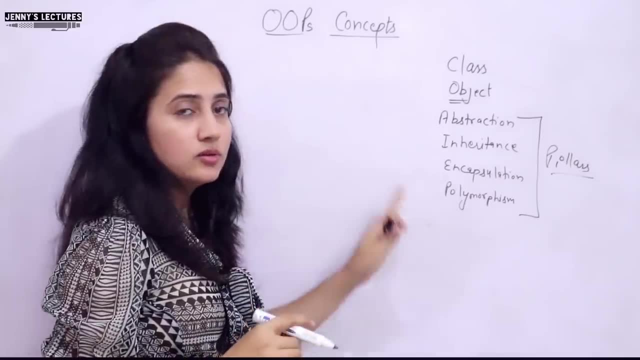 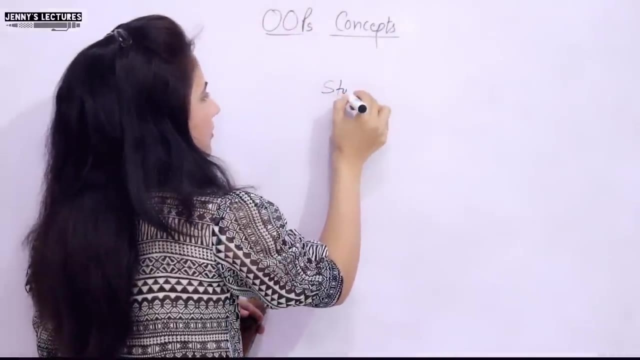 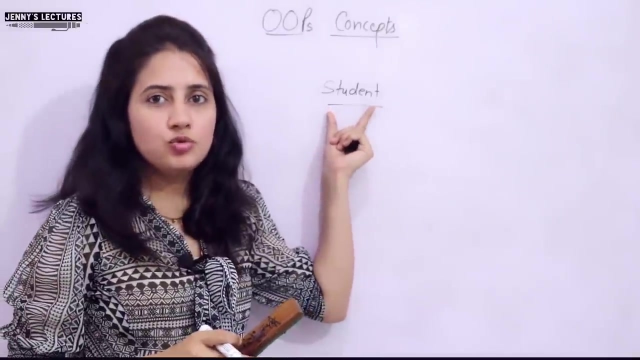 see these concepts and these four are known, as you can say, pillars, pillars of object oriented programming. but we'll discuss these six things, all these six concepts. so let me just take one example. see, let's take one example. like student maybe you will, you know, really related better student. so, simply, student in student in your class, you have male as well. 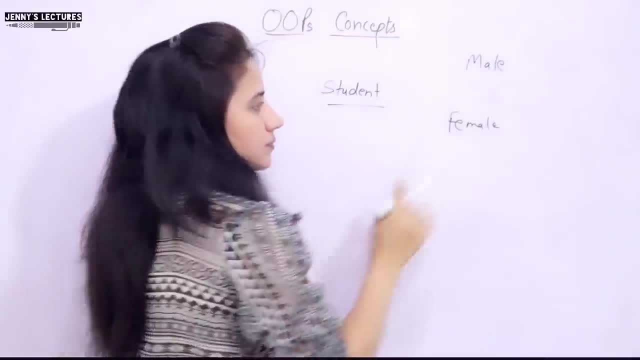 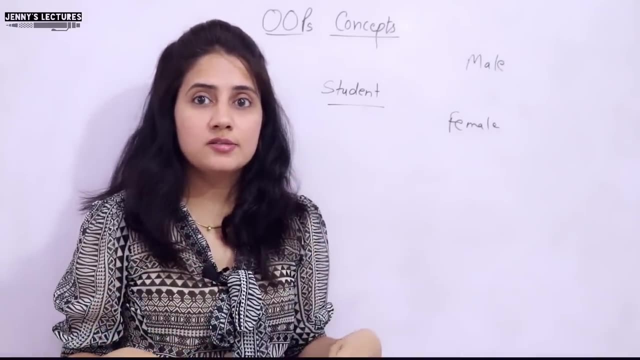 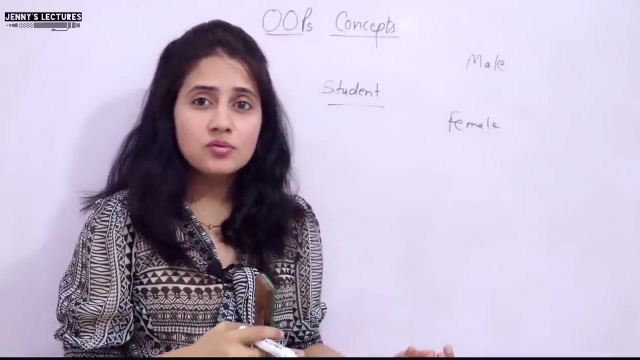 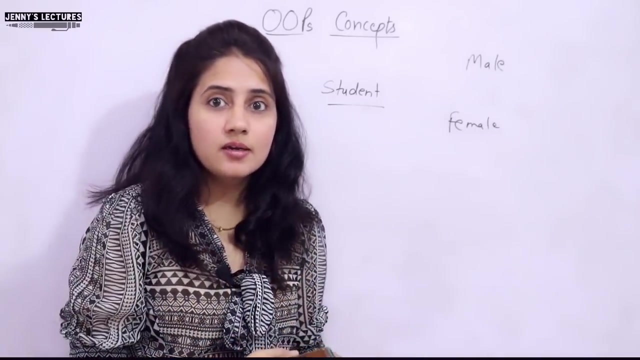 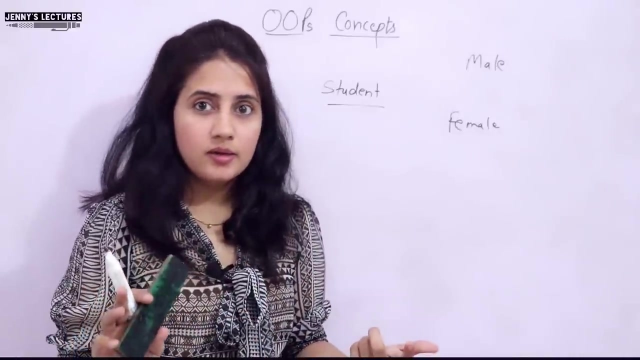 as female student right now. every student is having some common properties, like two hands, two legs, two eyes, nose, height, weight, color. these are some common properties they have, right. and some functions like slide, sleep, can eat, can study or speak and sit here. these are some common functions, right, every. 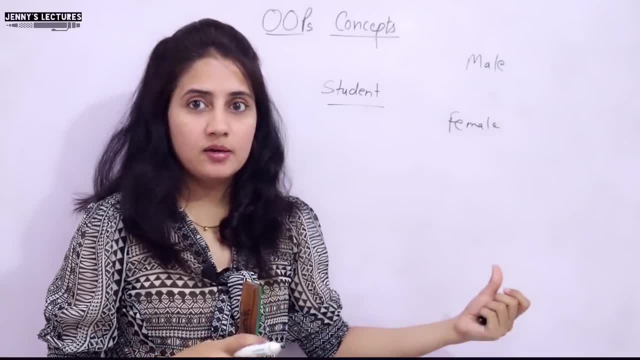 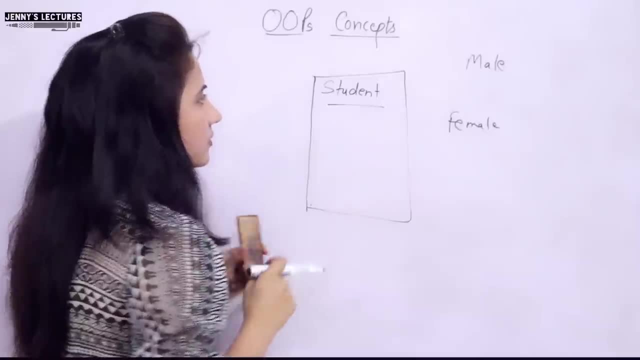 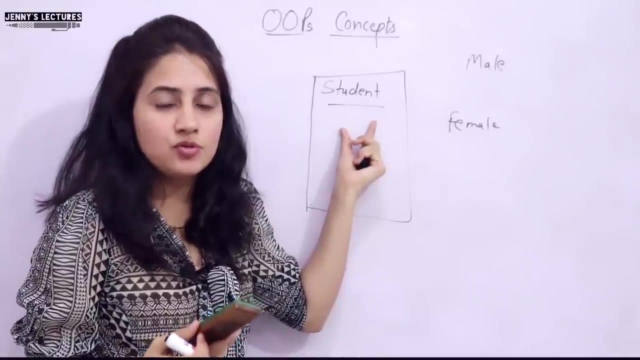 student is having either male or female, so we can consider it like a student is a class, which is what it is like. you can say a user defined data type in technical terms. if you say, then it is a user defined data type in technical terms. if you say, then it is a user defined. 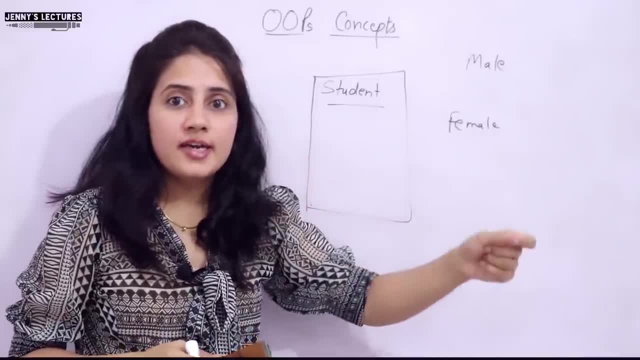 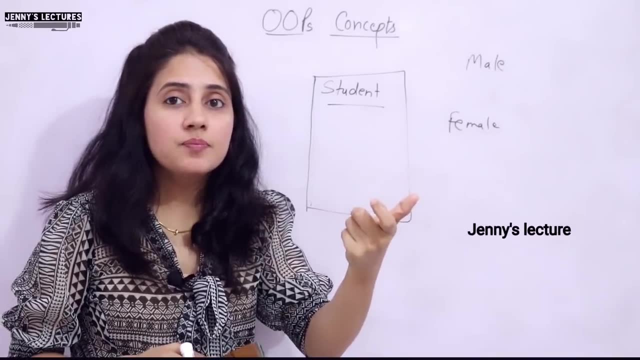 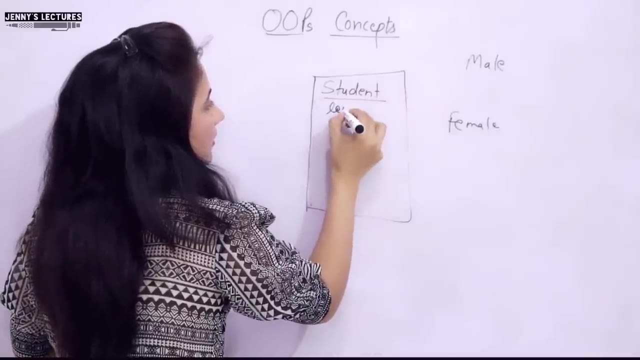 data type in the visual is just a user defined it like. as in see, we have structures, user defined data types, which is having some data members and member functions. now, what are those data members are attributes, the properties they have, like student is a class and having like. 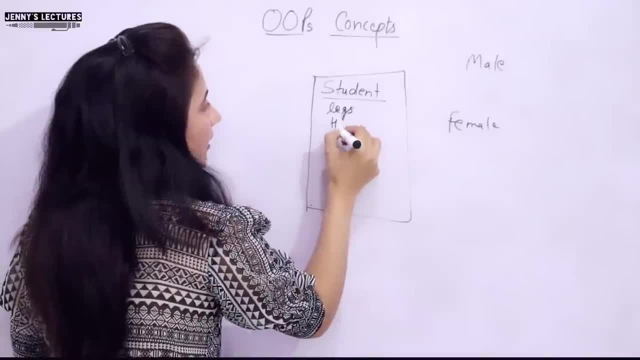 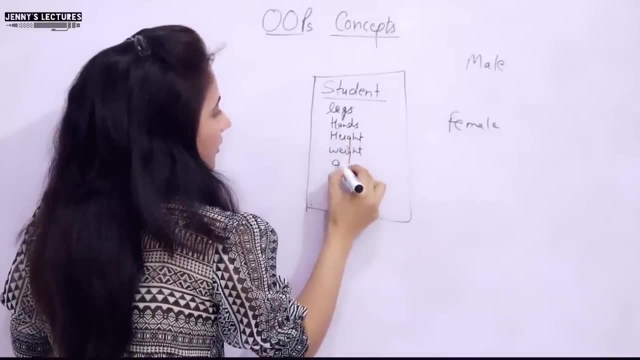 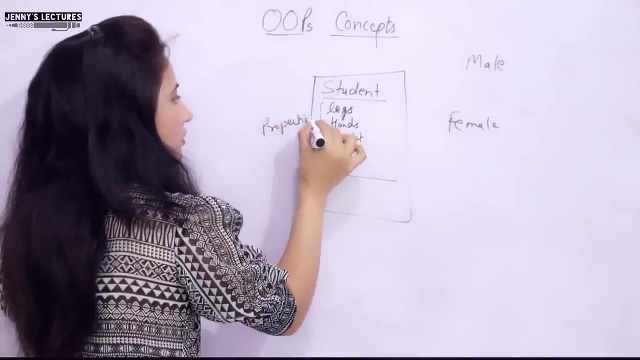 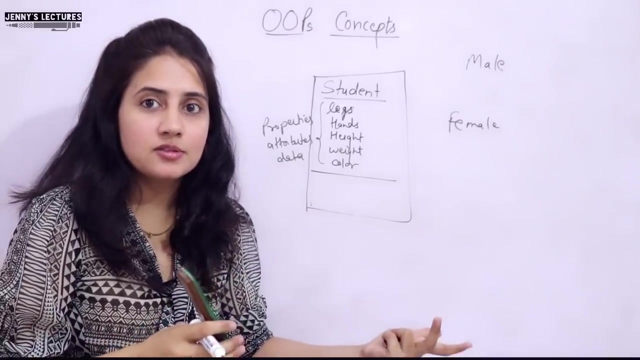 you can say legs and hands, some body parts you can say. then you can say height, weight and color. right, These are some properties, or you can say attributes, or you can say data, or you can say data members. So, whatever the data that would be considered as in the form of, that would be. 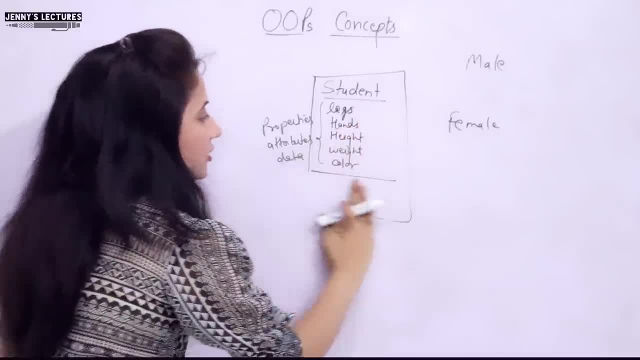 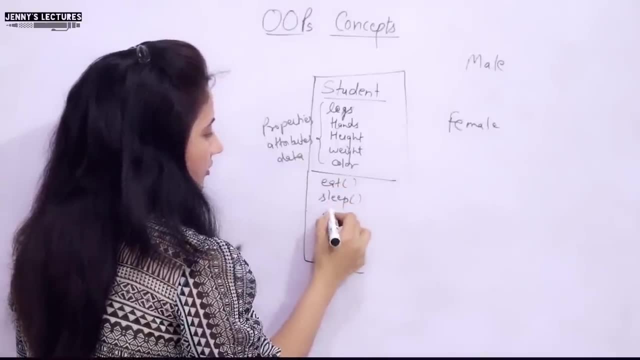 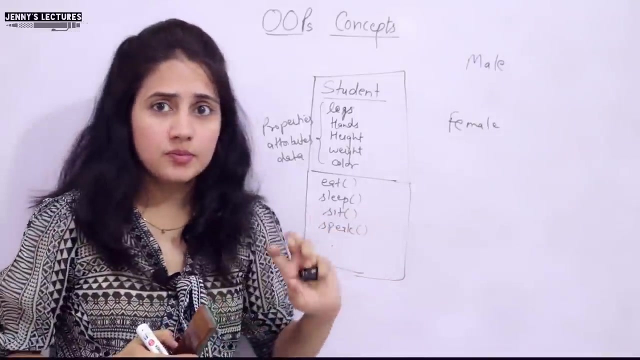 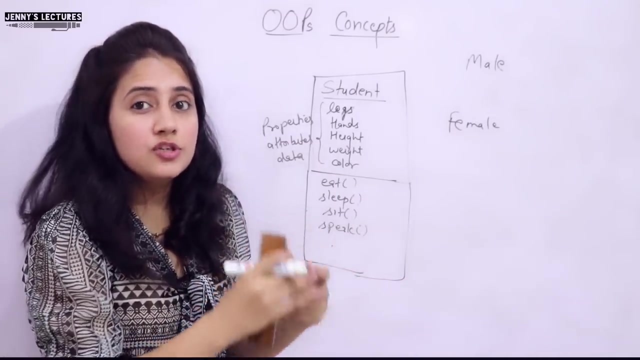 stored in the form of variables in the class. Next, functions what we can have like eat, sleep and sit, speak and many more. So these are some common functions, right? So class is basically what? a blueprint of an entity which defines the core properties and functions of that entity. 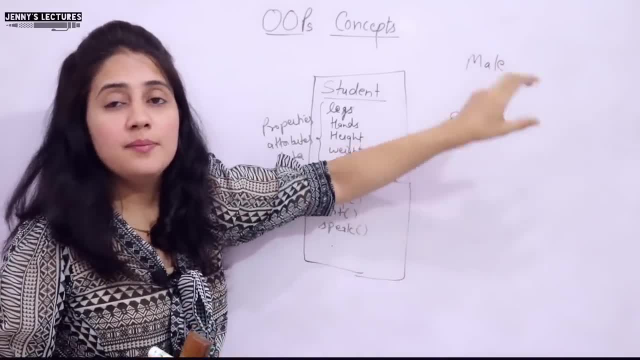 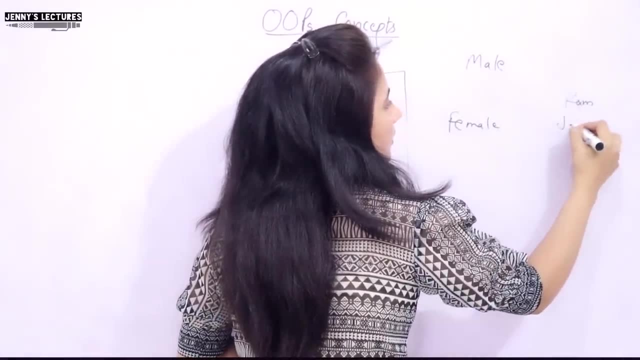 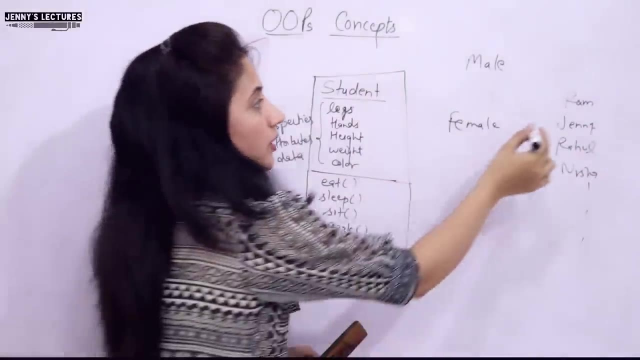 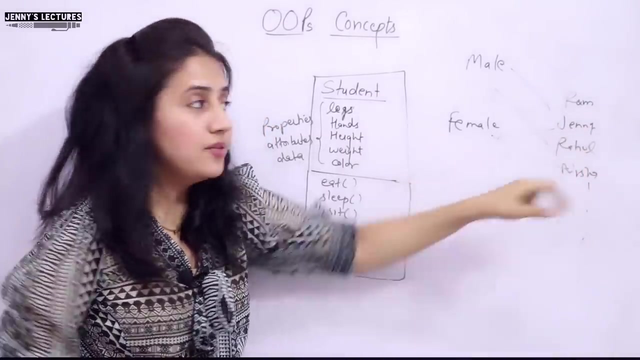 Now, entity means what Entity is male and female? you know, students, Actual students are entities, like student name can be Ram, you can say Jenny, Rahul, Nisha, These are some students. So male students, female students, right, So these are, and you can say real world entities and these are known as, known as objects. 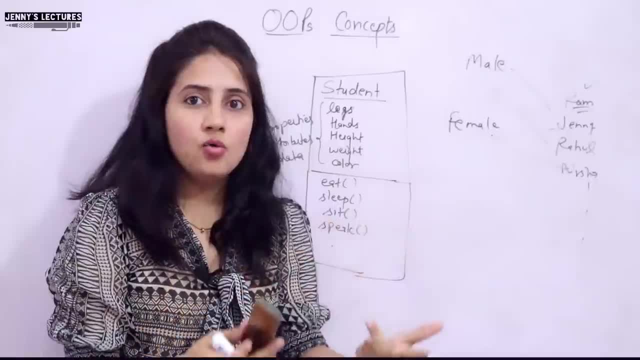 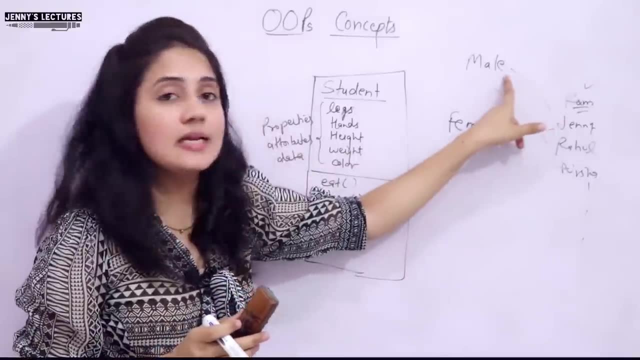 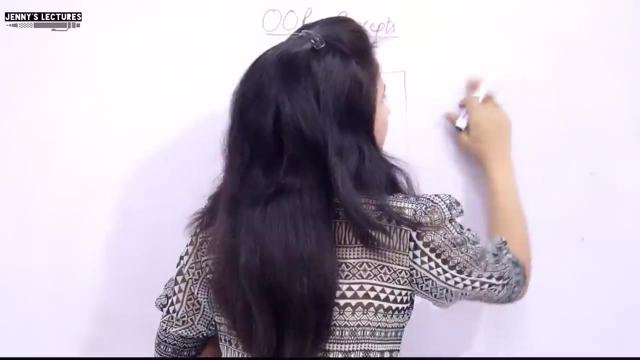 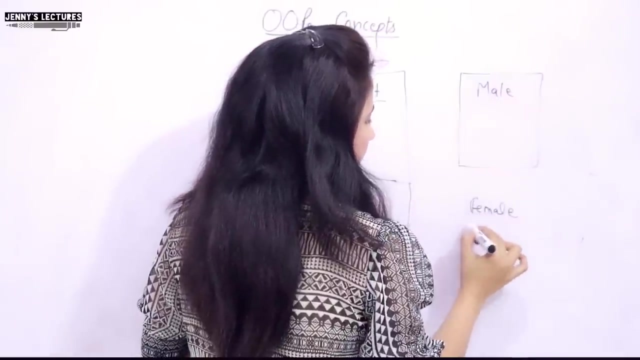 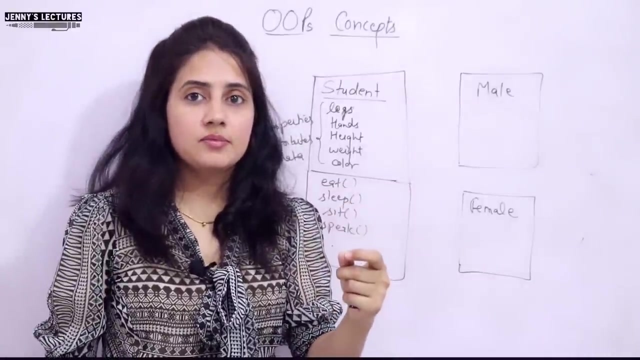 right. In my class I have a student like Rahul. Rahul is an object, right Of class, male class, Right. Two more classes are there. You can say like male and female. Here we have male, class and female. So object is what A real world entity, Rahul, physical existence, Rahul is. 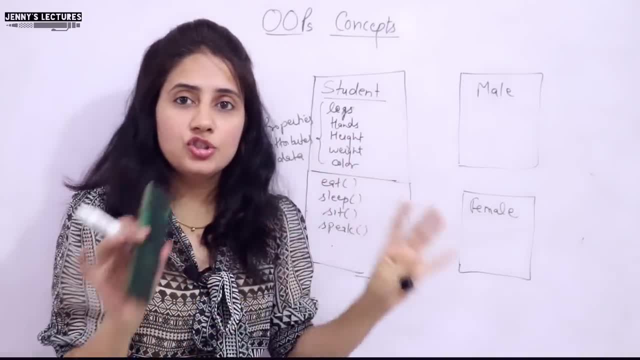 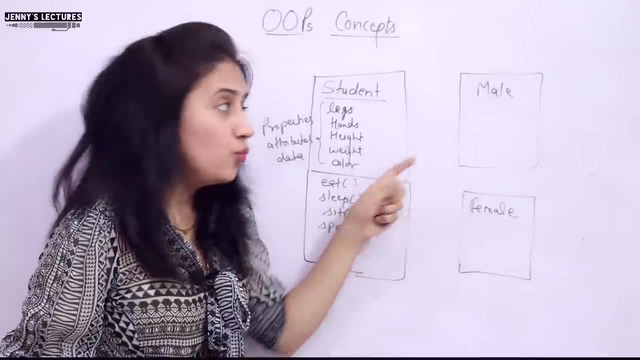 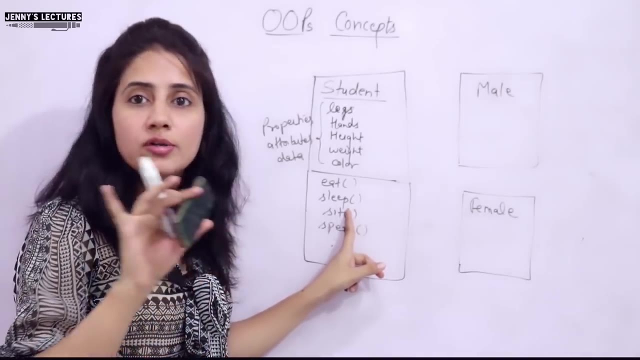 having physical existence. Class is just a logical thing, It's just a definition. You, it's just a blueprint. So no memory allocation would be done when you define a class. no memory allocation Because it is just a logical thing. it's not physical. Object is physical thing. 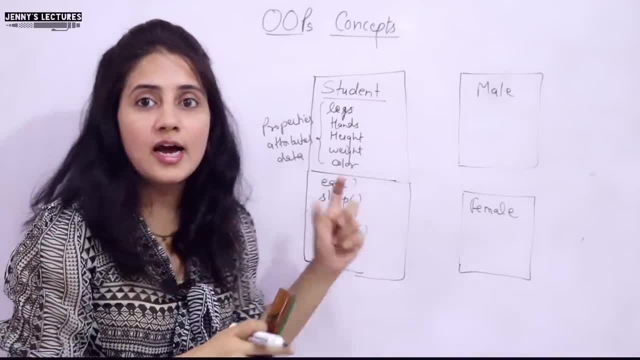 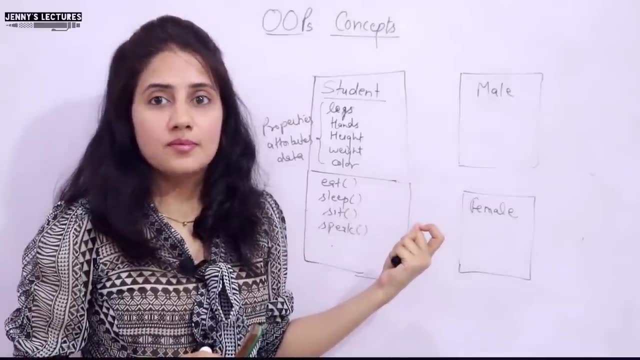 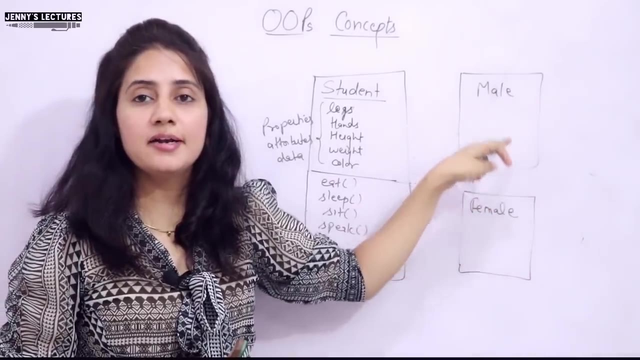 Now we can access these properties and functions of a class using objects of these class, or you can say instance of this class, right, Rahul is what you can say, an object of male class. So whatever is there in male, the attribute and the functions Rahul can access Using Rahul. 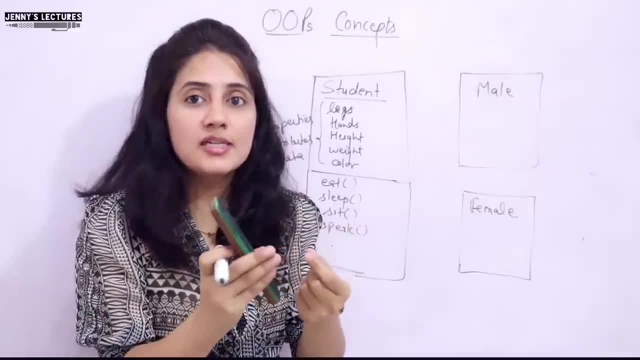 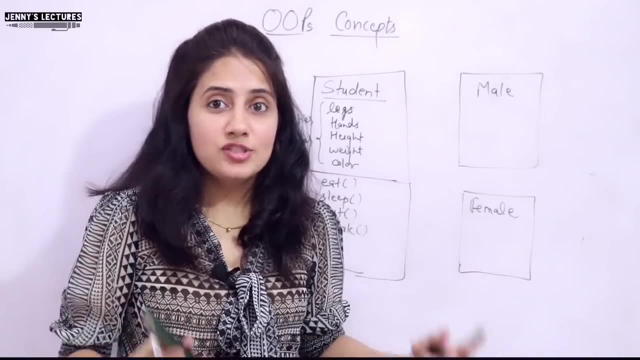 we can access those properties and those functions. So Rahul is physical thing, Rahul is having some space right In this environment, here in the class, right So same. when you create an object, then only memory allocation would be done in the 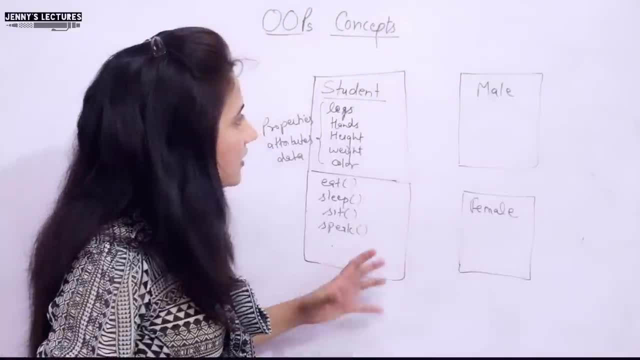 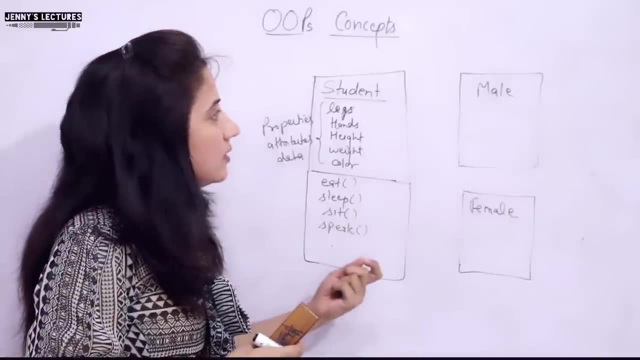 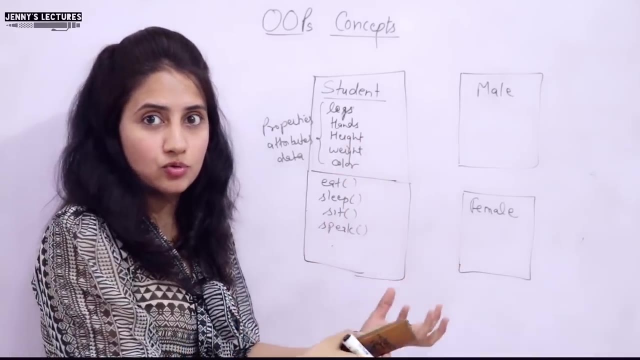 if I you know, say in the form of programming: So class is what It is, just a blueprint or a prototype through which we can create objects. or you can say it is, you can say group of objects which share common properties, right, Common properties and common. you can say attributes. 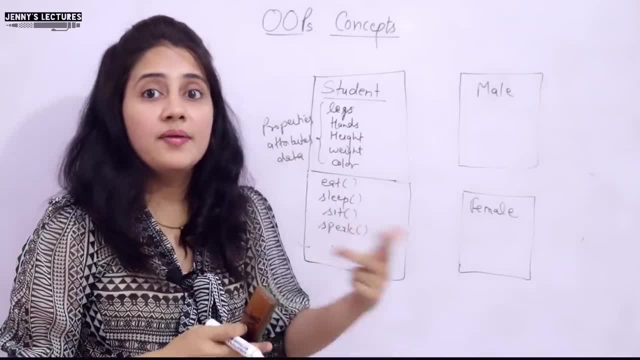 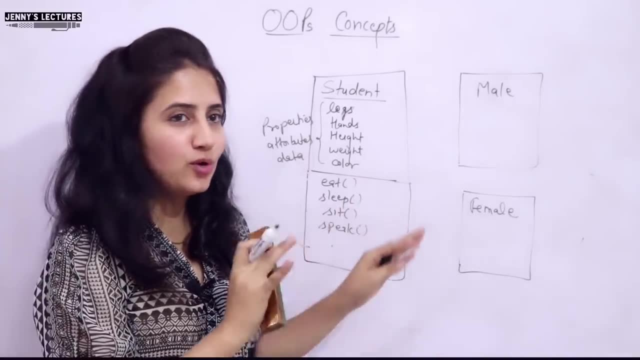 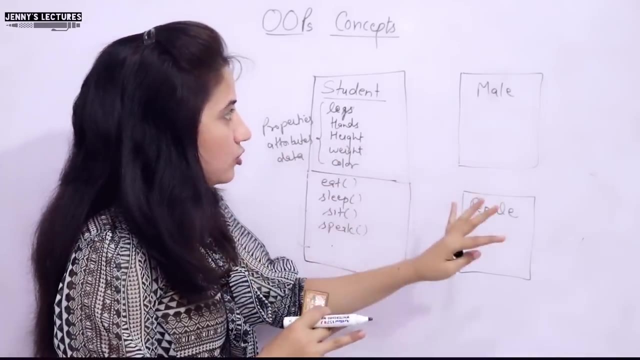 These are attributes. This is, you can say, behavior or methods. behavior or methods or functions. we can say: Don't worry, I have notes. also, I'll provide you notes. Everything I have written in my notes, Handwritten notes, right, You just have to understand now, right, What is class and what is. 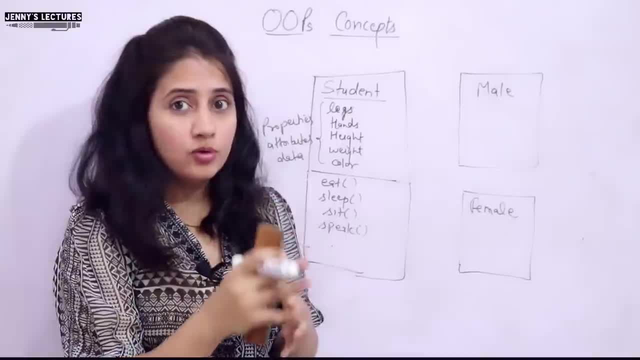 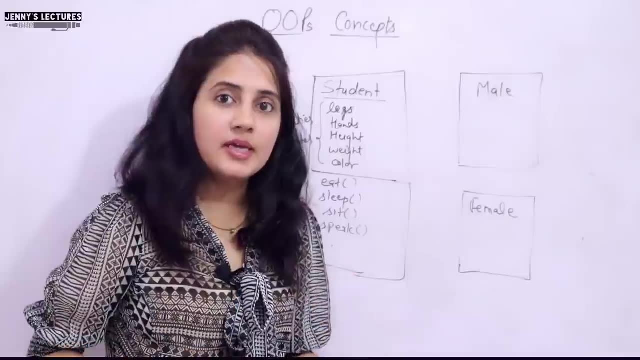 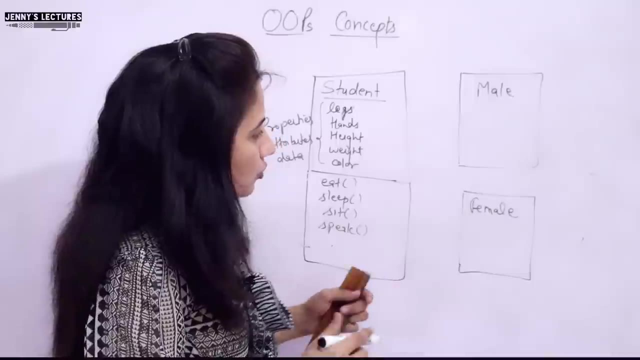 object. Now see object also. I hope you got it right. It is a physical thing or it is a real world entity, right? Which is having some behavior or some properties of its own behavior and properties. fine, That is object. So like suppose I have an object. one object is Ram. 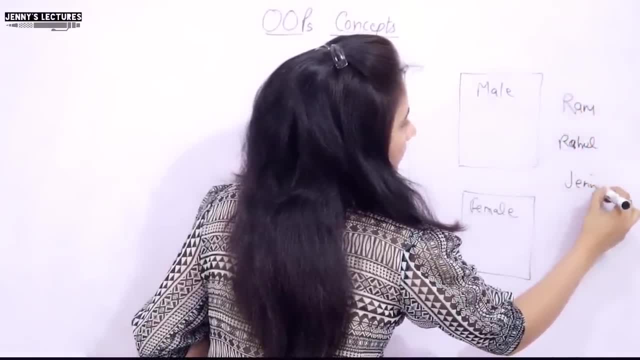 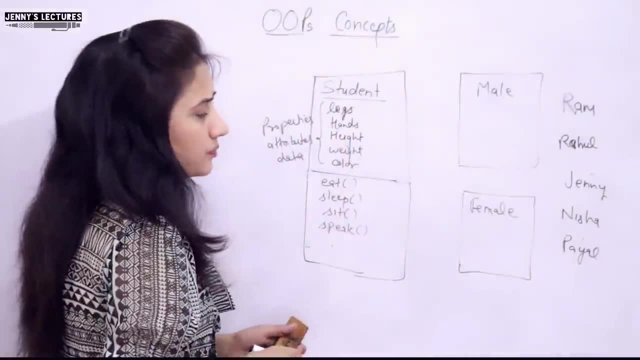 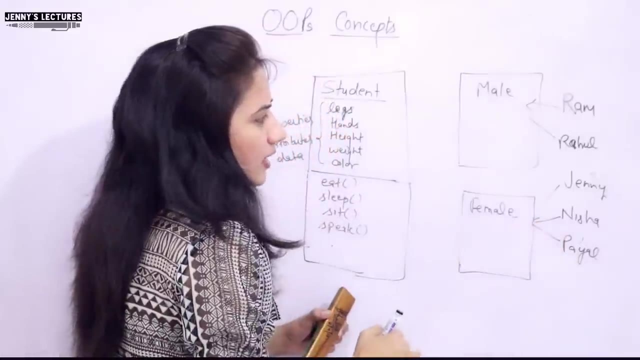 Rahul, Jenny, you can say Nisha and Payal, These are some objects, right? So objects are just an instance of a class. Rahul, these are instance of male class. Jenny, Nisha, Payal, these are instance of female class. So they they are having their own data and functions, or you can. 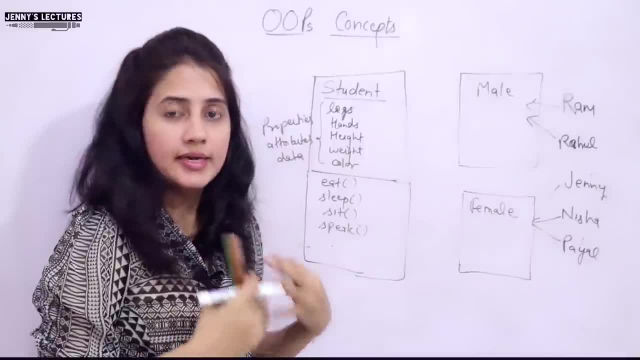 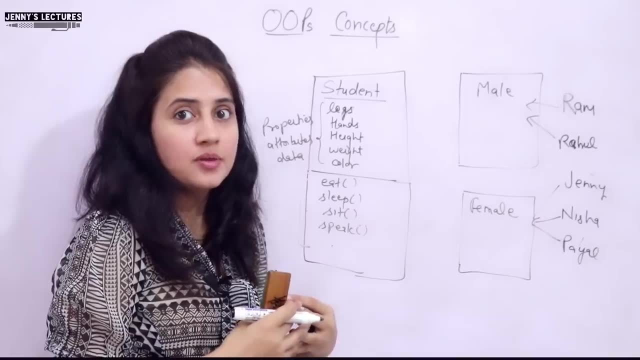 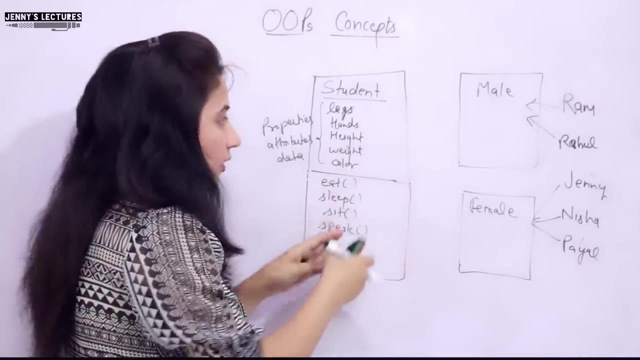 say the code, right, Each object is having its own data and the functions- The functions are which can manipulate that data. Each function has its own function and data, Like Ram, is having its own. you can say height, weight, color, right, And on function is there, Ram is having its own. 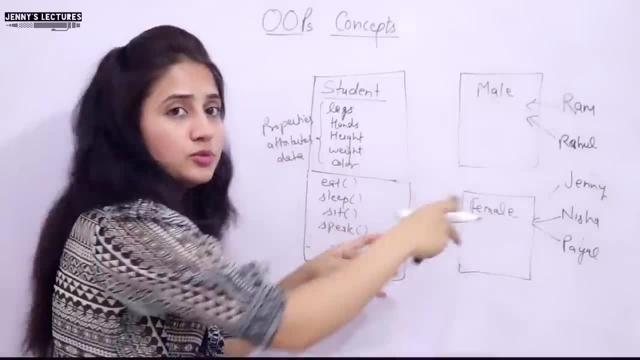 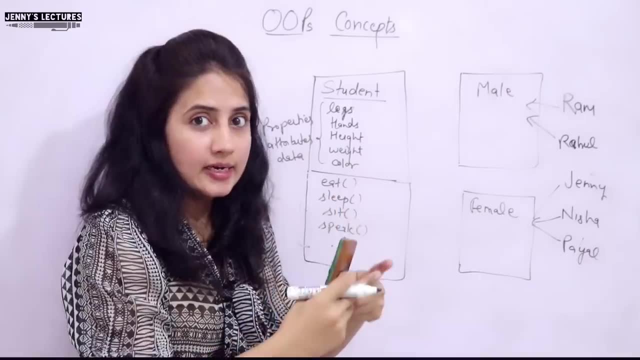 functions. Rahul is also having different height, color and weight. Every object is having its own. you can say code and data. Using code or the functions, we can manipulate that data fine, And each object can interact with each other with the help of message passing. 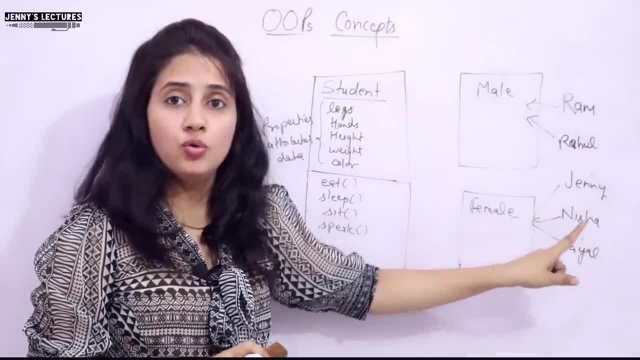 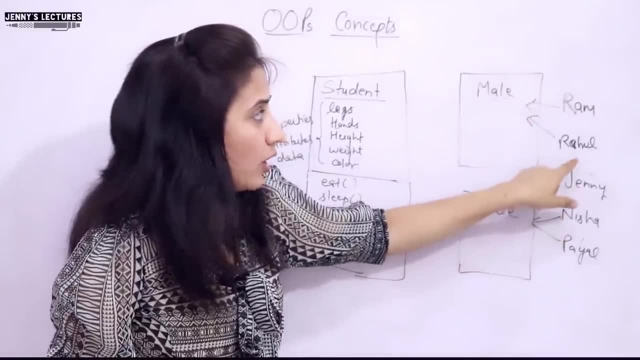 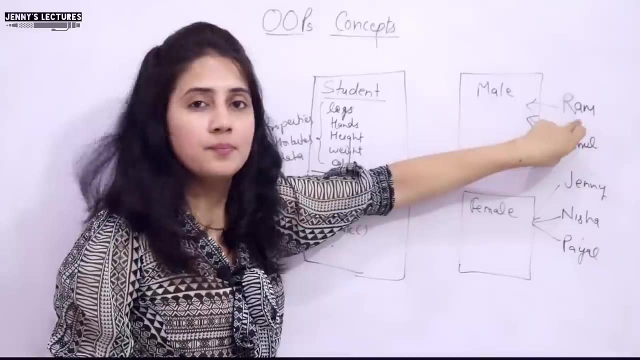 And for interacting, they don't need to have the internal knowledge of their data and code. Suppose, if I want to, Rahul want to communicate with Ram, So it's not like that Rahul has to know the internal everything about Ram, right? What Rahul need to know? In which form the message? 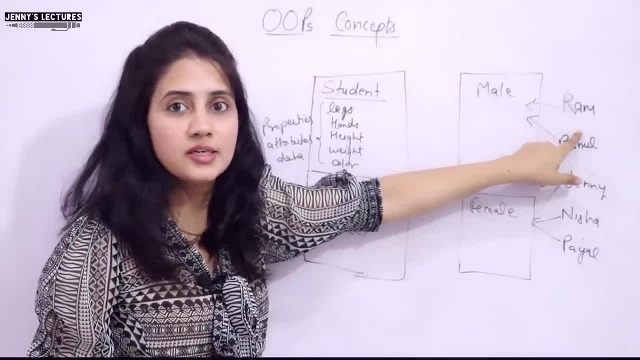 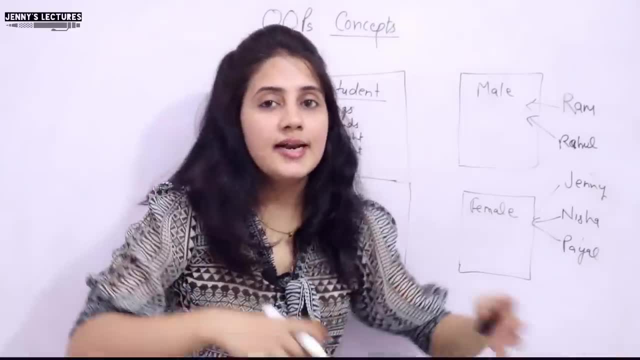 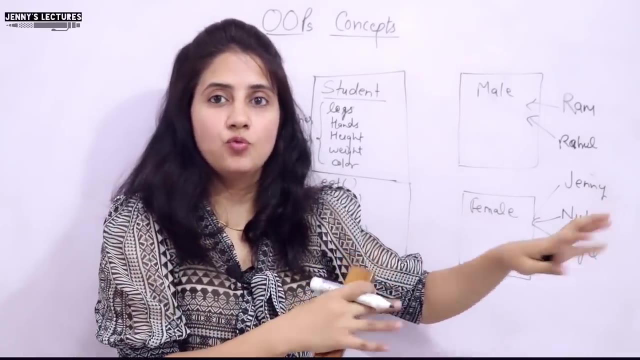 would be accepted. or you can say the language Rahul understand- Hindi or English- that's it. And in which language Rahul will respond, that's it. So same in programming, one object can interact with other object without knowing the internal detail, the code or the data of that object. What just need to know? The type of 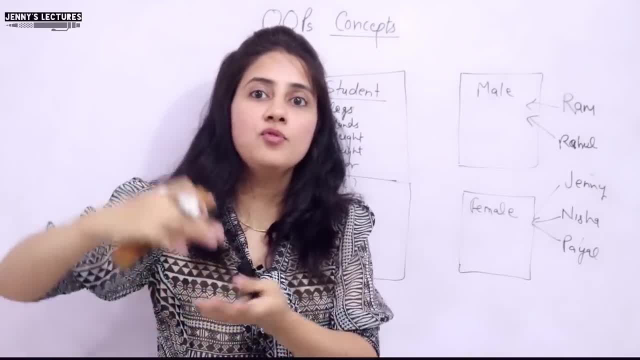 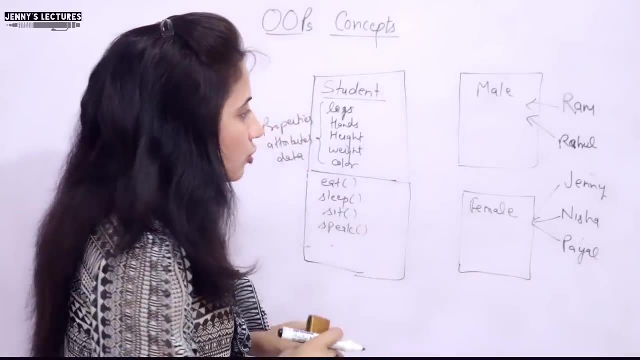 message would be accepted by other object and what type of output, what type of response that object will give right. So the objects can also communicate with each other using message passing. So class is just a logical thing. It's just a blueprint. a blueprint to create a class. 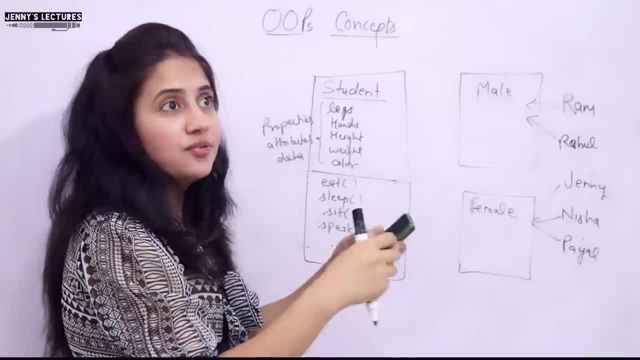 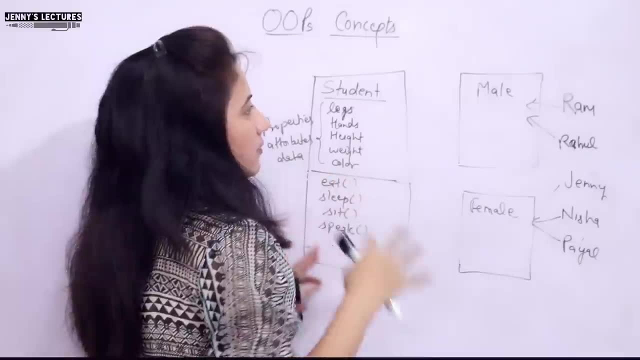 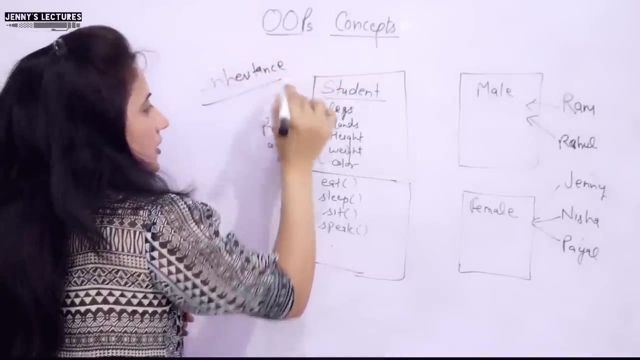 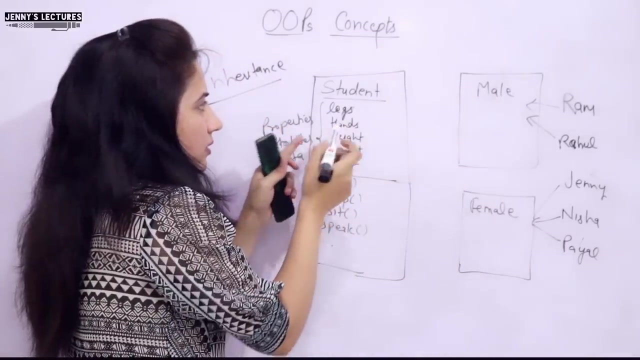 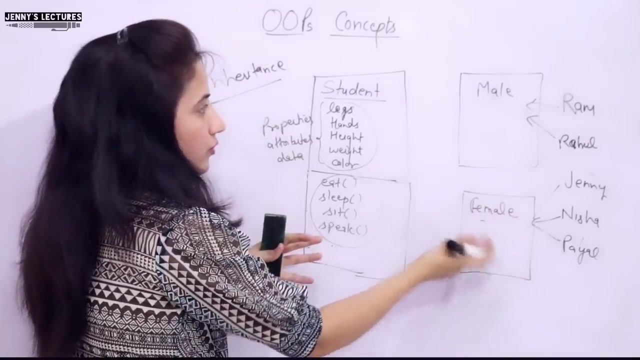 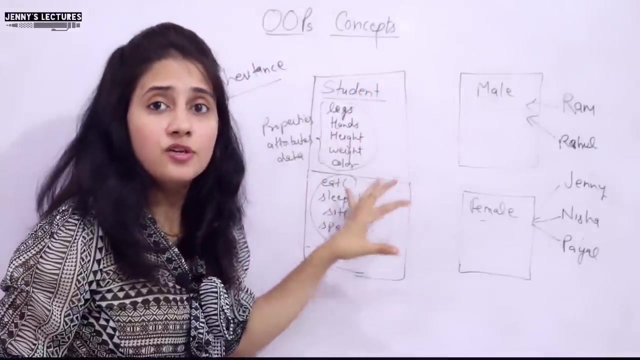 So this is for question and answerunknown process. Their and female will also have. female in a student will also have these properties and functions, and these properties and function we have already defined in a class student. so rather than defining these things, rather than defining these functions and everything here also, here also. 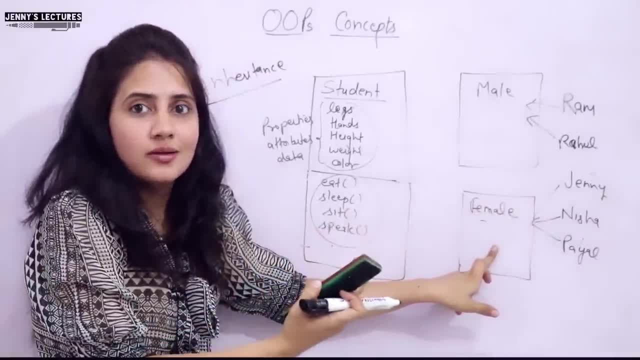 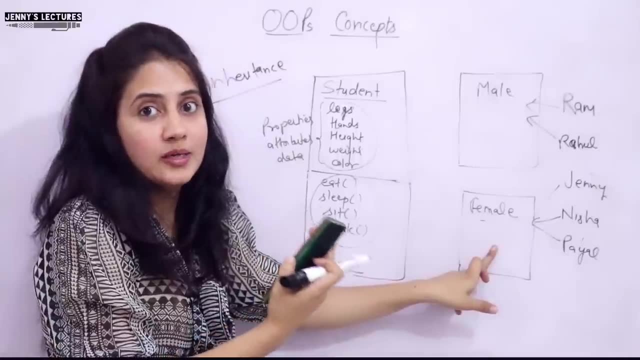 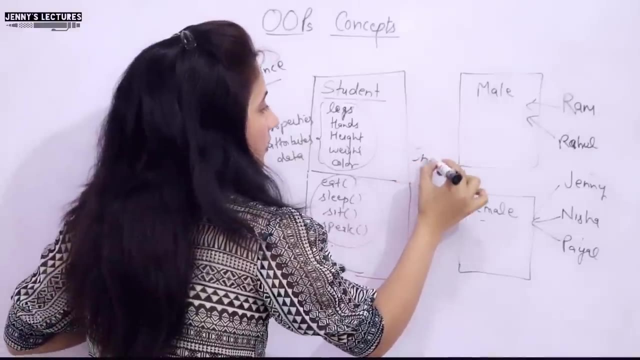 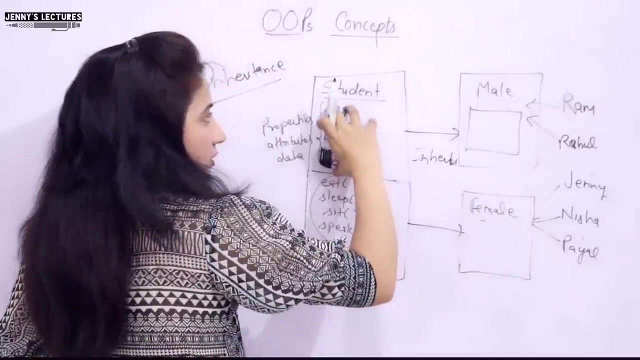 we will do what. we just reuse this thing and how you can reuse. this is one of the most important characteristics, or you can say pillar of oop oops. you can inherit these properties through inheritance, so they will inherit these properties here also and here also. so whatever is there, these 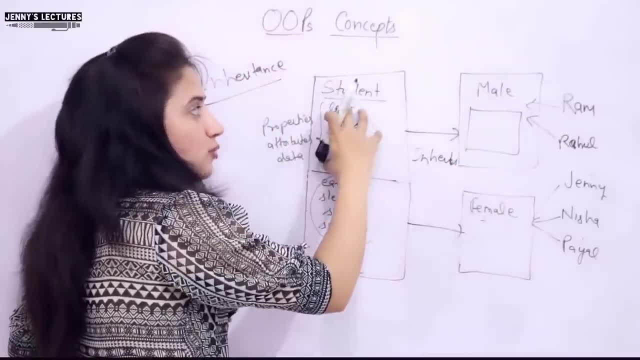 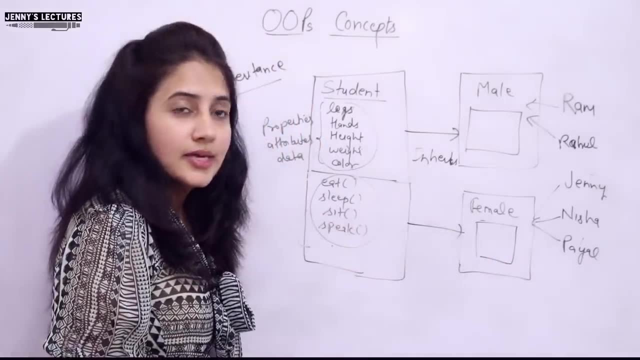 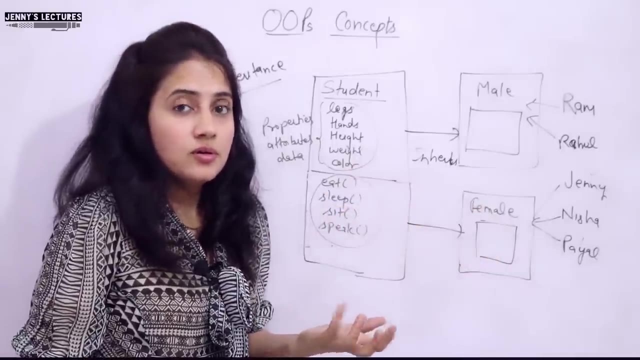 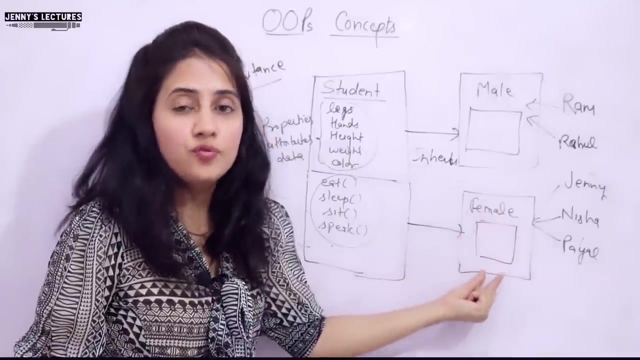 functions. you can say these functions and the attributes. attributes means the variables and the functions. right. here also, and here also. and male and female, each class can have their extra, their own attributes, like some body parts in female are having which male are not having. so they can have their own data, their own function, right. 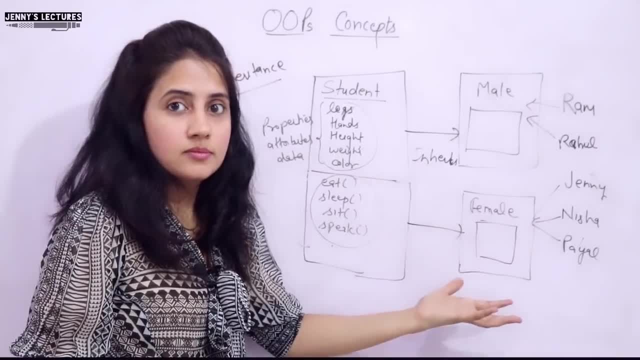 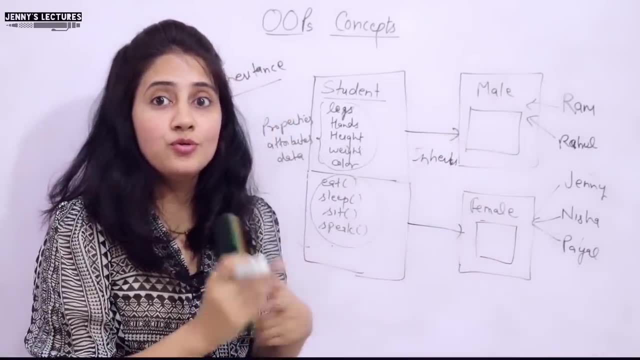 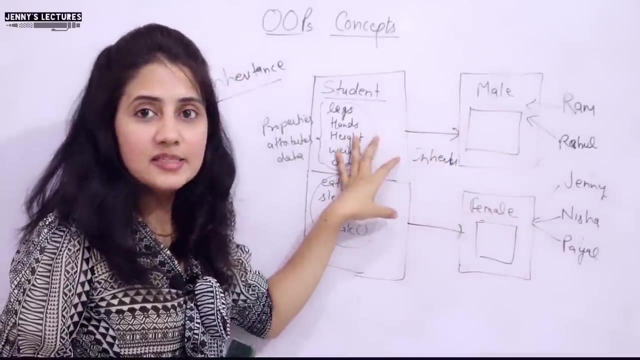 male can also have their own function and data and thus common properties. they can inherit from this class, from this class, rather than rewriting again and again. so this is what beauty of inheritance. these are known as child class and, what you can say, derived classes. in this class you can say it is first class and second class and this is known as. 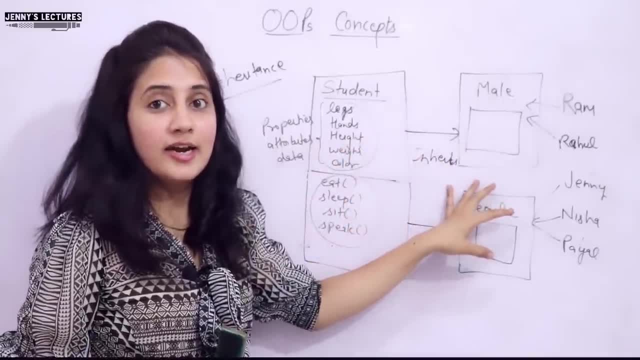 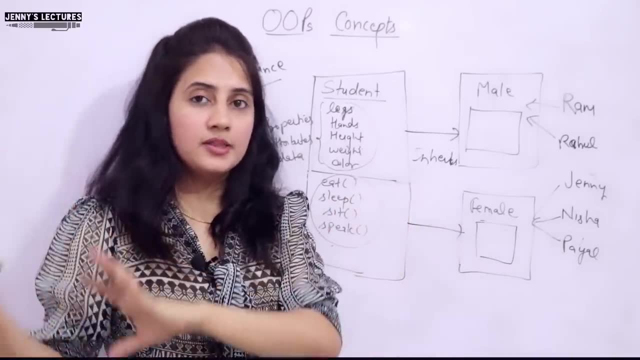 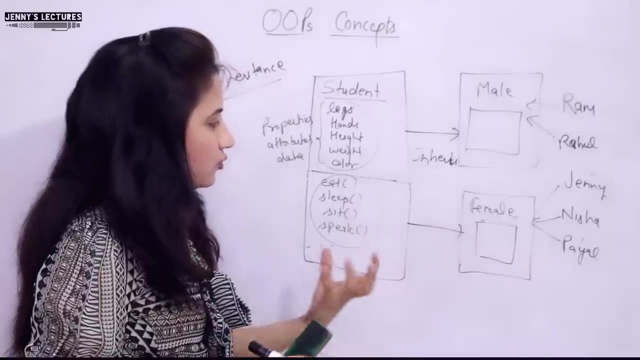 base class or parent class, right. so code reusability is there. so that is why, rather than writing same code again and again, productivity would increase. we can reuse some other code and we can just do whatever we want. we want to do one more thing in object. i want to tell. in technical terms, we say: 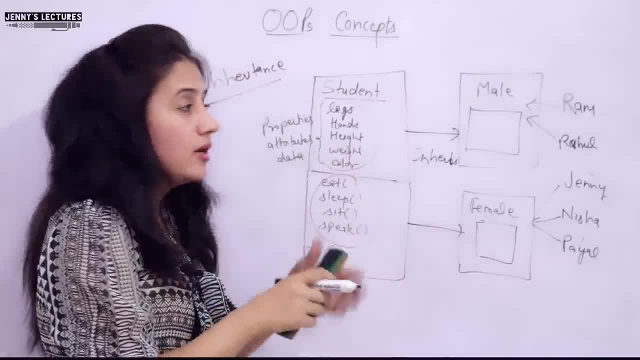 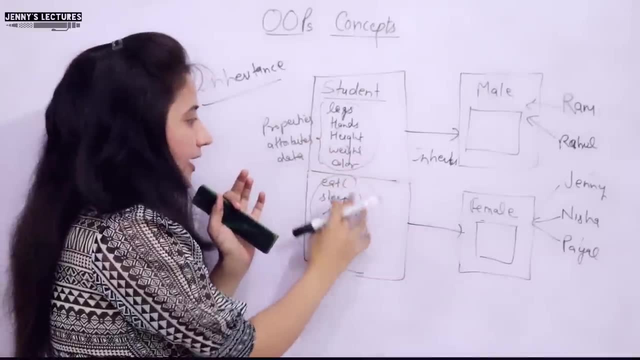 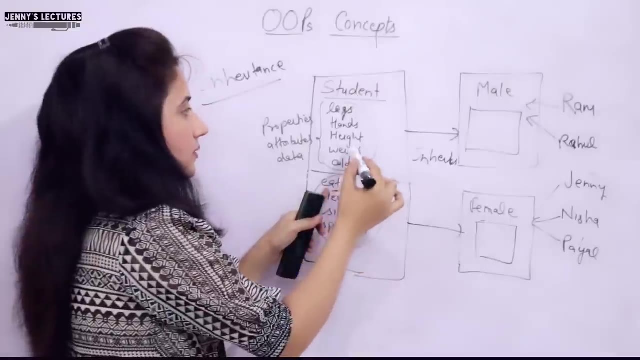 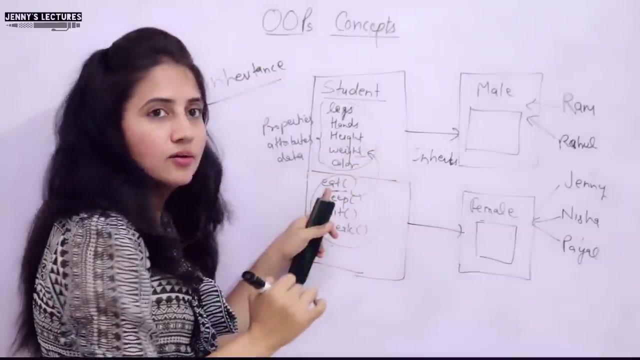 objects are having its own data and code through which we can manipulate the data. like ram is having data and code, means the functions, this code right, whatever we write here. so if Ram- suppose I can say if Ram will eat more, then weight would increase, so through these functions we can modify these data of that object. it's not like 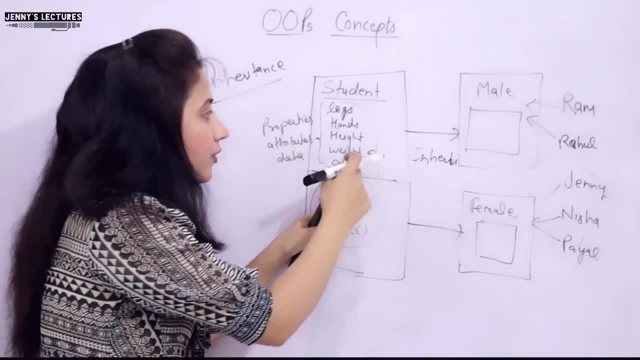 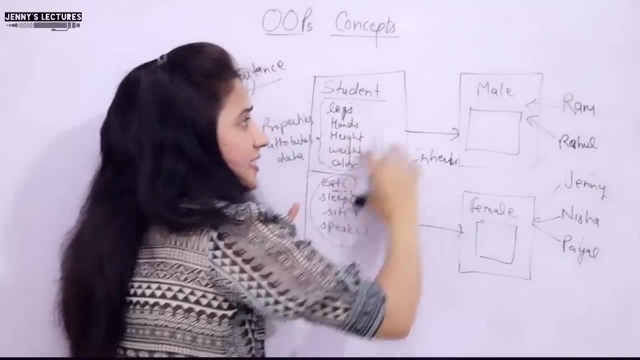 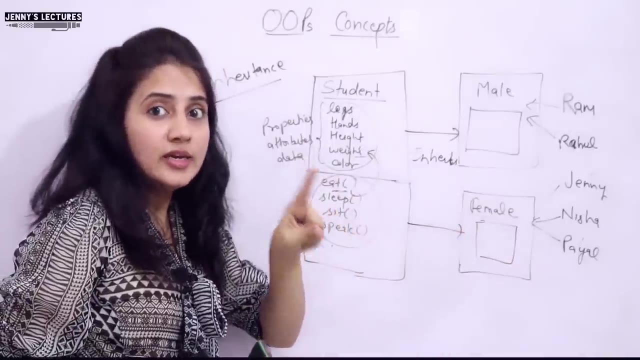 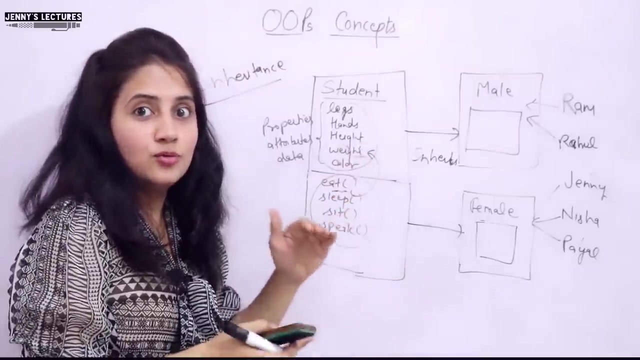 that if Rahul will eat more, then weight of Ram would increase. no, because these details are specific to these objects. if Jenny will eat more, weight of Jenny will increase, not the weight of Nisha or Payal right. so this data and code are binded together in the these objects. using that code, we can manipulate the. 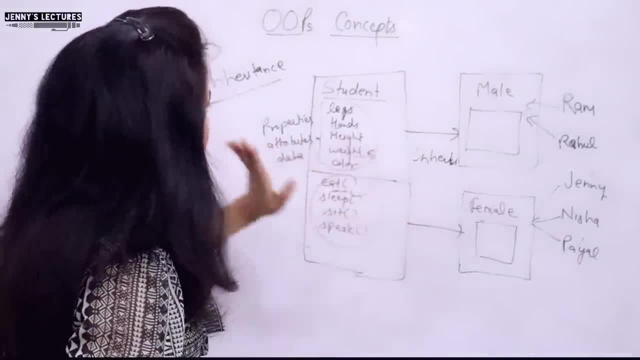 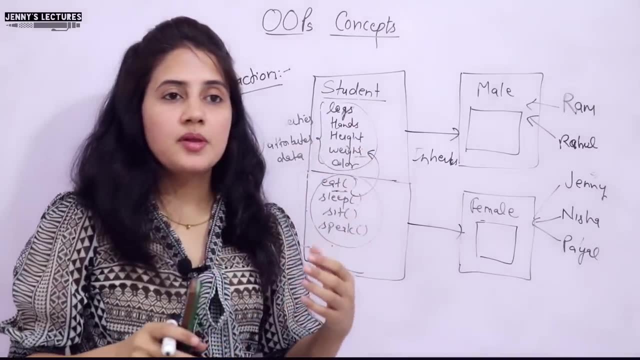 data of that object. finally, I hope you got class of objects and inheritance. now we will see what is abstraction. see, let's take one example first. suppose there is a coffee machine. what is there? one button is there: make coffee. you just press this button and 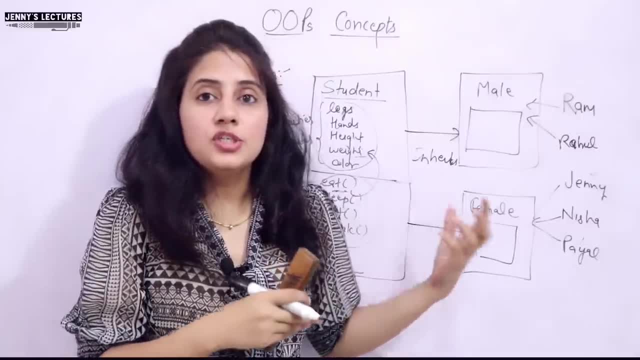 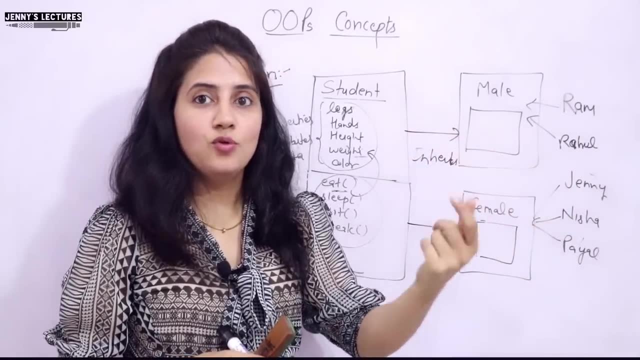 your coffee is ready. right, if a machine, second machine- is something like that. there we have a button like add some cold water to the pan, boil the water. second button works, but in the second one it does not work right now. if a second button is like this or like that, than I add some water to the pan, boil the water, after that add new water. 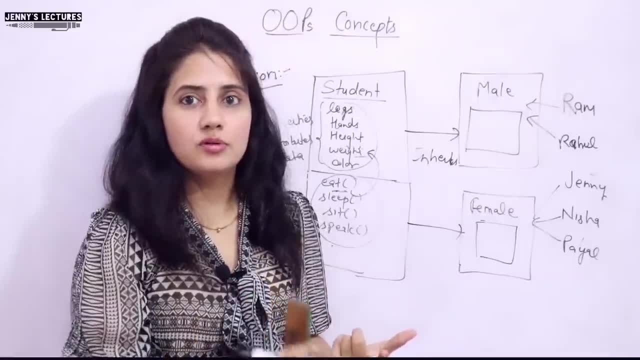 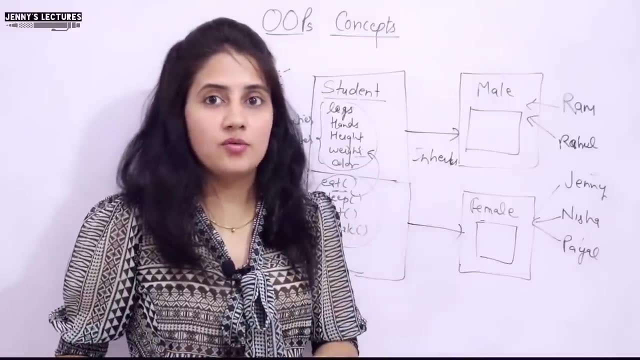 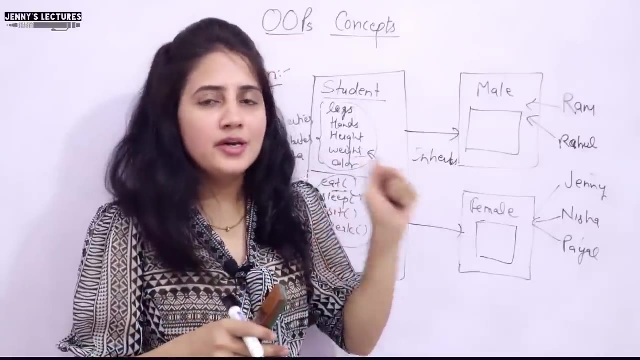 is: boil the water. third button is: add one cup of coffee there, add sugar, this, something like this. we have many buttons, the complete process we have right. so which one is better? just the first machine, having one button make coffee. you just press this button and coffee is ready, you don't. 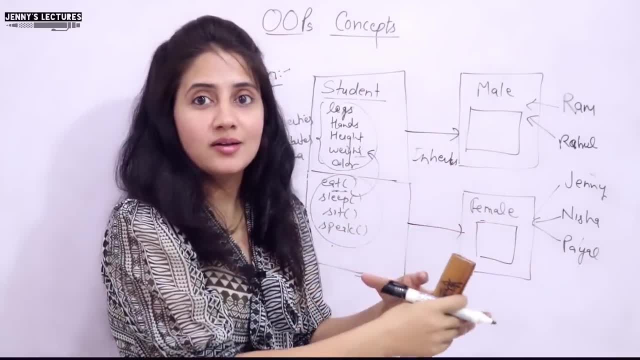 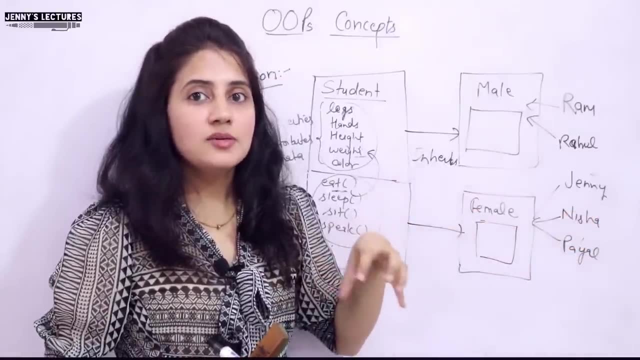 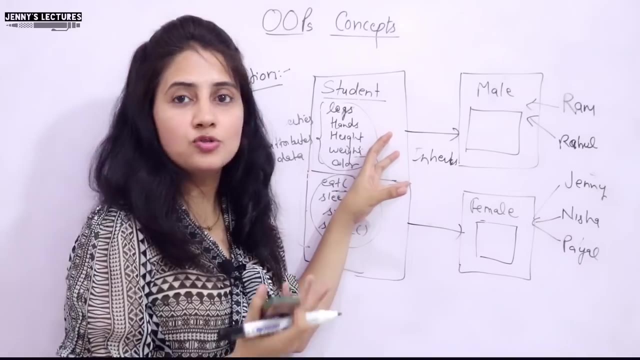 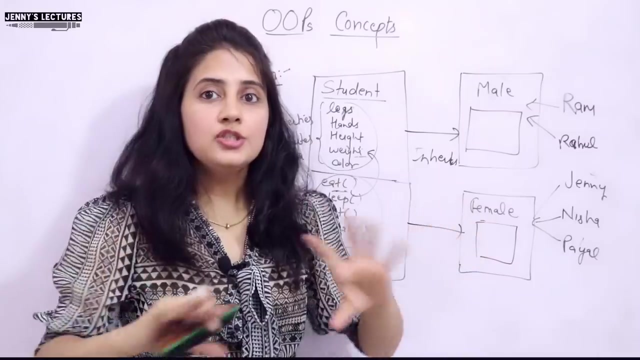 need to go into the detail. the implementation part means the making part of that coffee. right, so means in first machine. we are just hiding the detail, the process of making a coffee from the user. that is what abstraction, hiding implementation detail from the other world only showcase the relevant details, which are relevant to the world, which are relevant to the other users only. 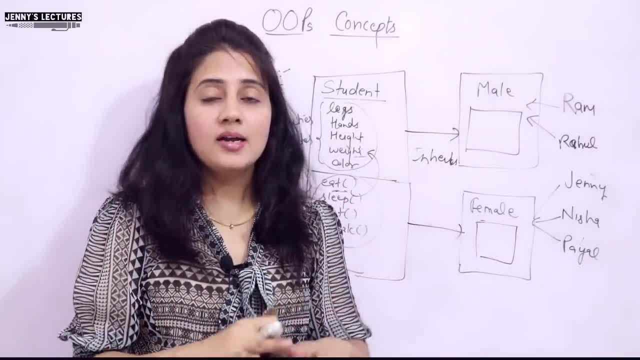 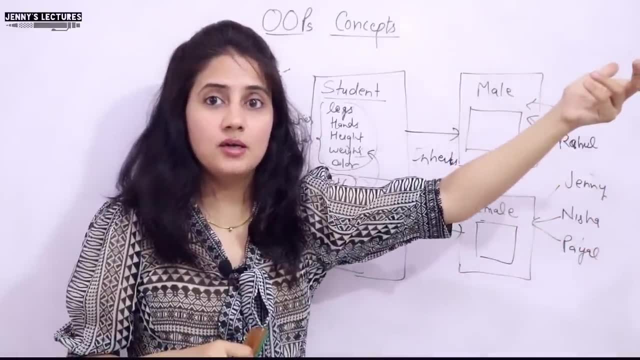 showcase those details, hiding the implementation detail. that is just abstraction, like when you switch on your fan. you don't know what is happening behind there. you just switch on, you just press that that button and your ac is on, your fan is on, your tv is on, like your dvd player. 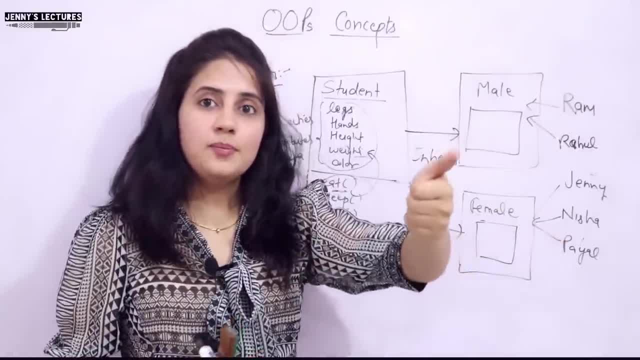 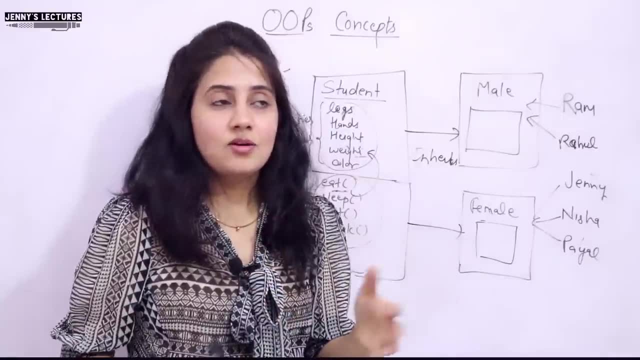 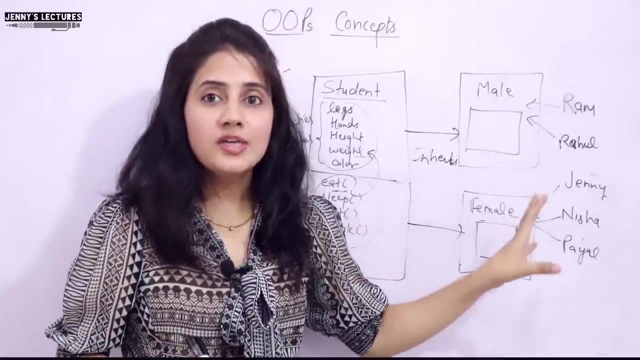 once you switch on your you know you can say the tv and the dvd player, or that you can say what is that set of box. then on the screen, the whole world is in your room. you can see everything right, but behind the scene what is happening? how you are getting that data on your tv, on your you know. 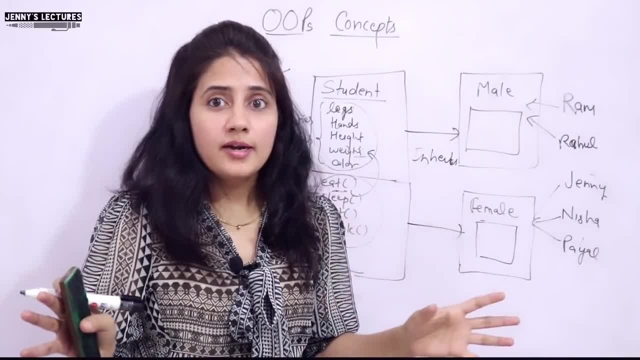 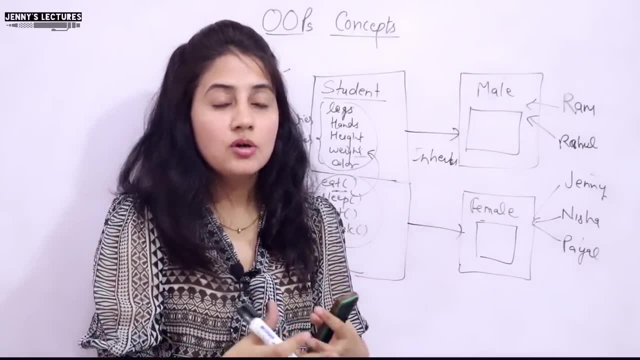 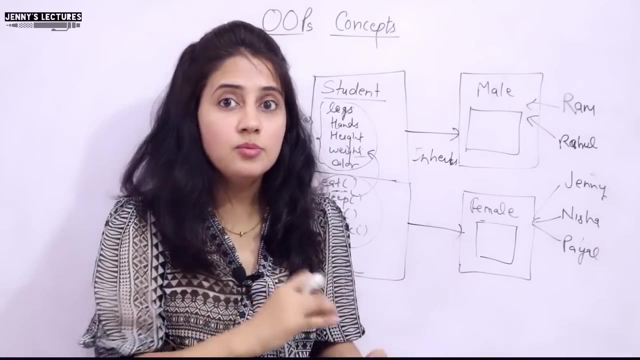 set of box through satellite or what is happening, you don't know, right. so that is what abstraction? same, hiding something into a function. or in java we can- uh, you can, we can- achieve this abstraction with the help of interfaces and abstract classes. hundred percent in abstraction we can achieve in java, right, so hiding something into a function. 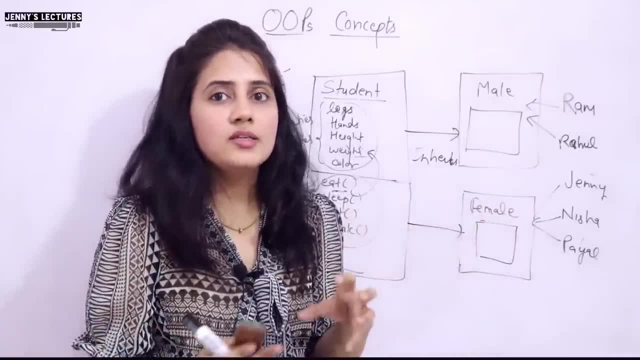 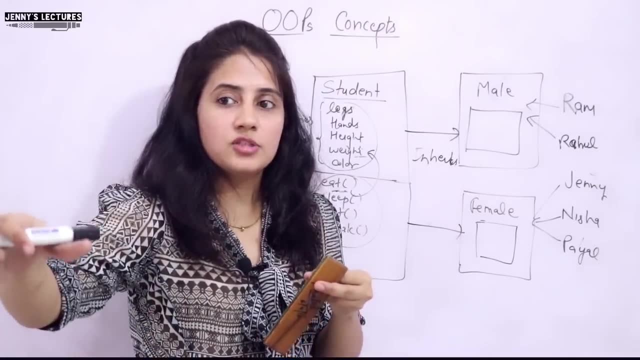 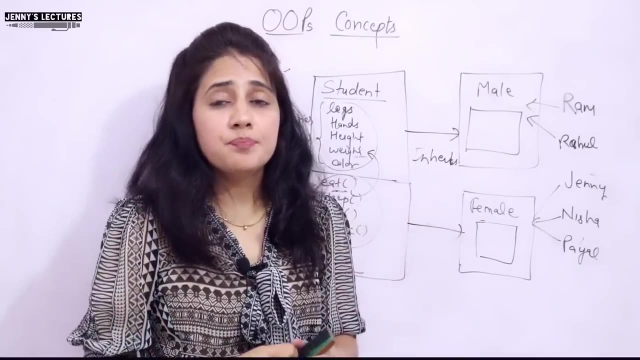 or you know, an interface, these kind of things. that is called as abstraction, because when you call a function, sometimes you don't need to go into the detail of that function, that how that process is doing, you just need an output. you call that function and you need the output, that's it. because, see, there are in large scale application. 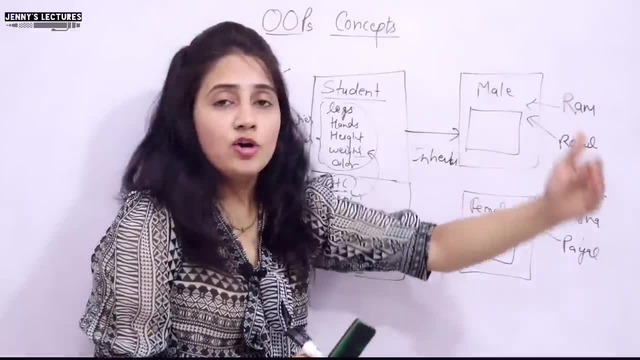 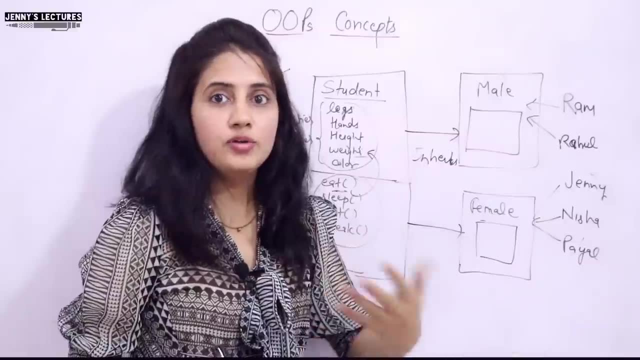 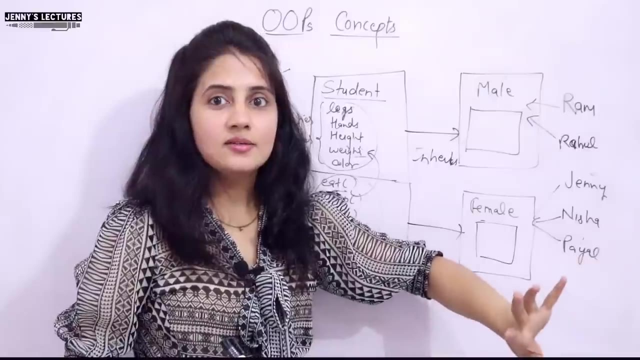 there's a large code base. if you go in the detail of each and every function, then it would take you even months to read out all the functions, and you would. you would never code right. so, rather than going into the implementation detail, just showcase the relevant details only. that is simple abstraction. 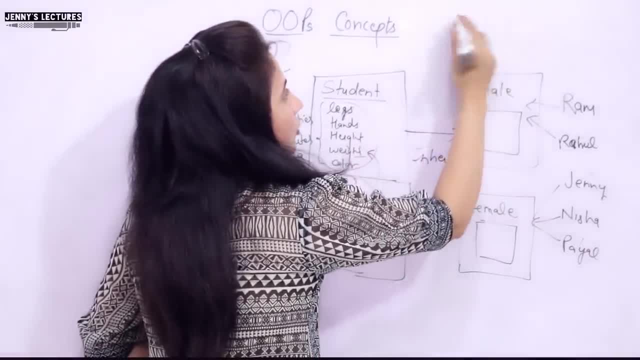 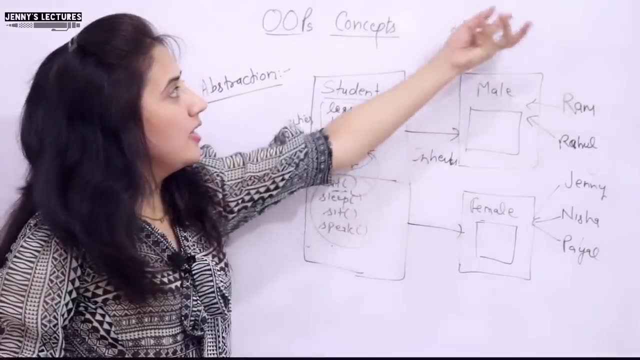 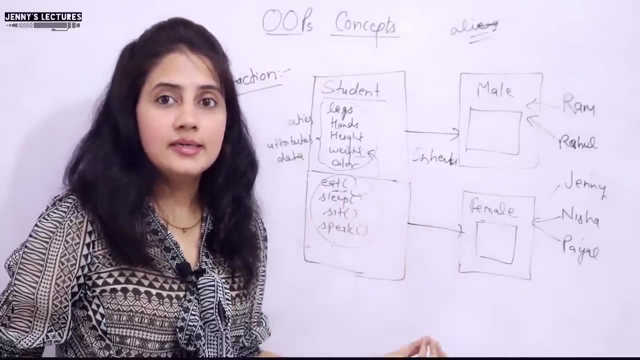 like in this, you can take some other classes, their animal or you can say alien- i hope spelling is correct. maybe animals or aliens know that like student or male and female can walk, can uh, eat, can do these kind of things, but how they don't know. the implementation detail. 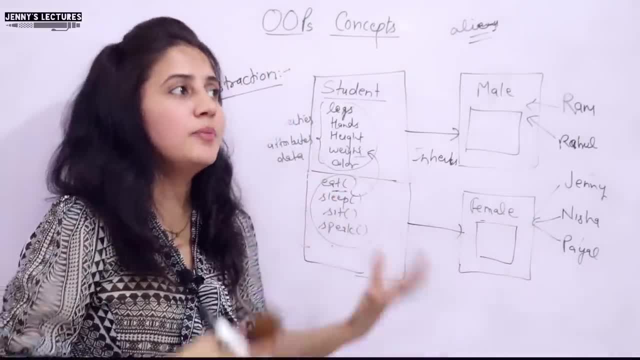 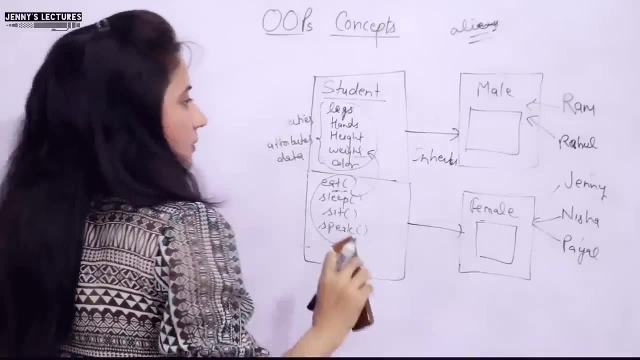 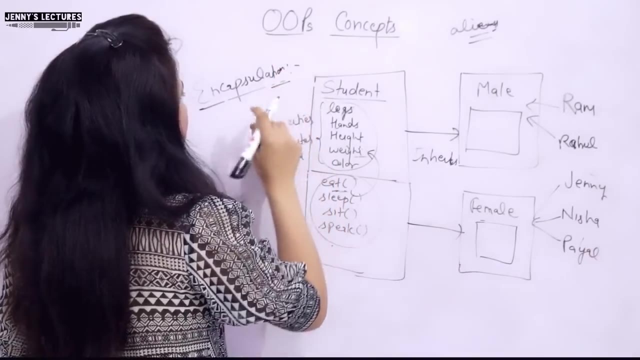 so that is simply obstruction in programming. also we can achieve abstraction, but how we will discuss later. just i you know. i just want to get you familiar with these terms, basic terms. next is encapsulation, as the name suggests, in capsule. capsule means means uh, you have uh. 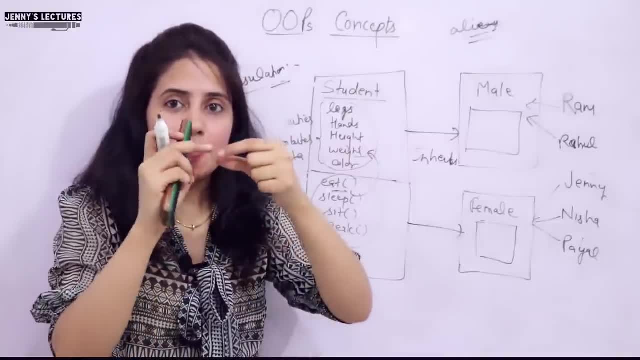 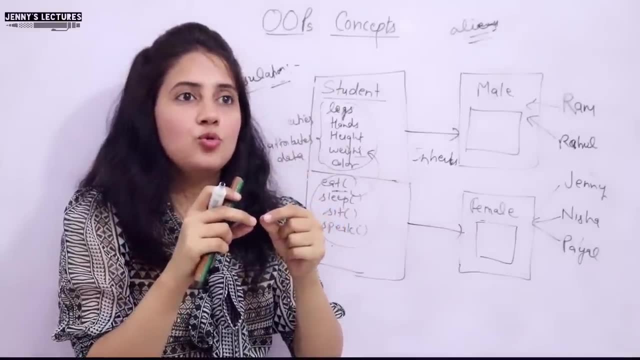 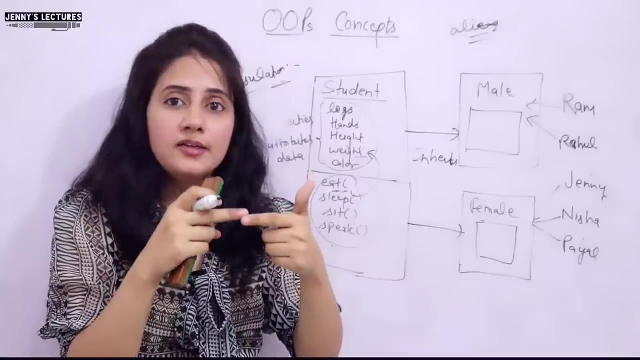 seen a capsule, capsule medicine, the tablet. there we have a wrapper in which we have some medicine, right, there is a wrapper around that, that thing, right? so that is what we are hiding: the inner thing we are hiding from the whatever is there in the capsule. we are hiding that thing. 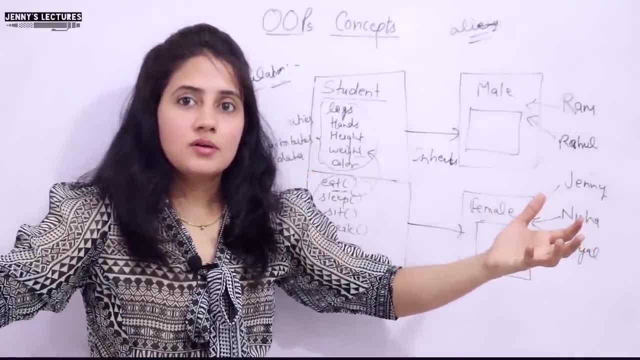 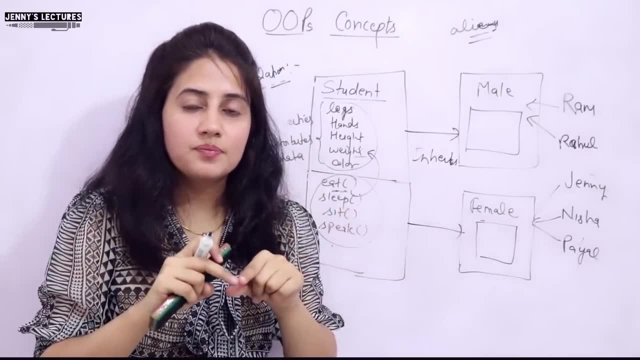 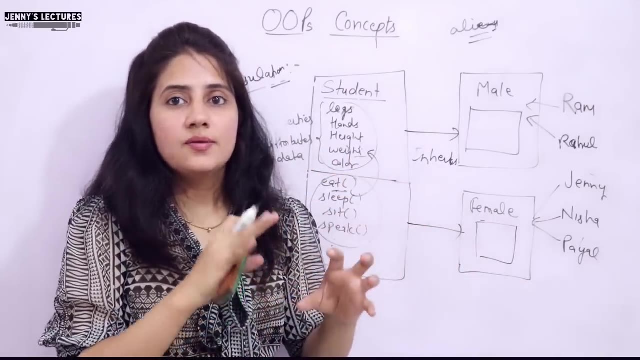 by putting the wrapper from outside the world. right, like around the chocolate we have a wrapper so that chocolate is hidden from the outside world with the help of that wrapper. right? so sometimes encapsulation is also known as referred as data hiding. right. so wrapping up of these. 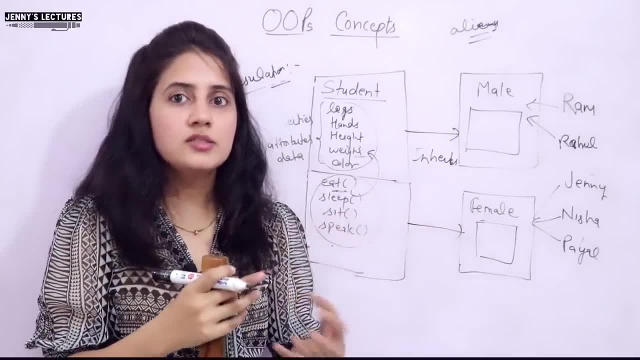 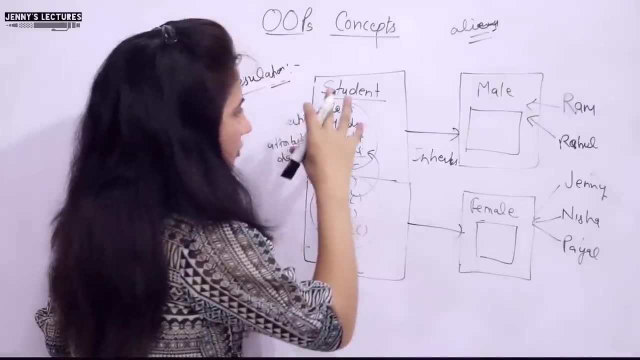 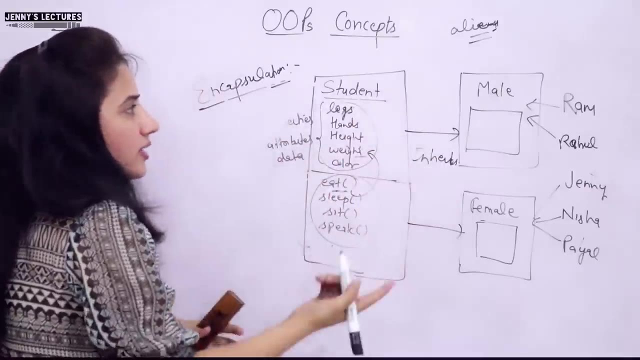 things- data and the functions- into a single unit. that is known as encapsulation. or you can say like something like this: you can take this example: binding this, this, you know, data and the code together in one unit is known as encapsulation. so simply, what encapsulation we can say like: 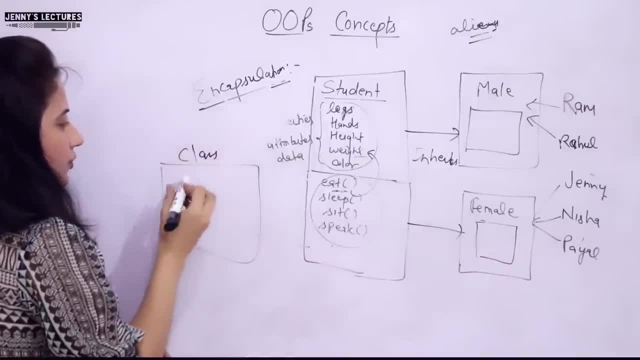 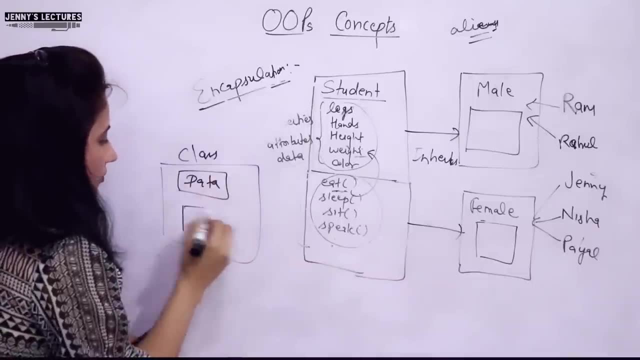 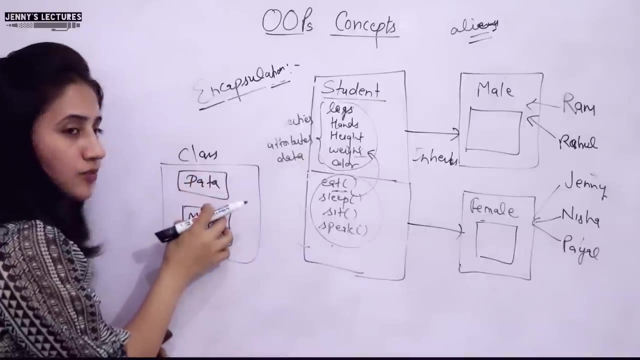 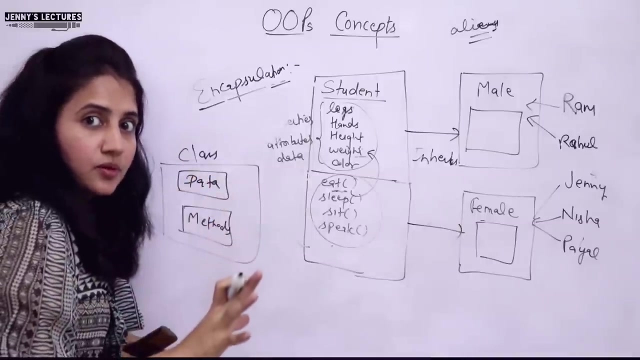 here in a class. this is a class in class. we have you, we have data or attributes- you can say right- and we have methods or functions or behavior, so binding these data and these methods or the functions together. this is known as encapsulation in c++. that's it, this is encapsulation. right now, you can hide this data from the outside world. 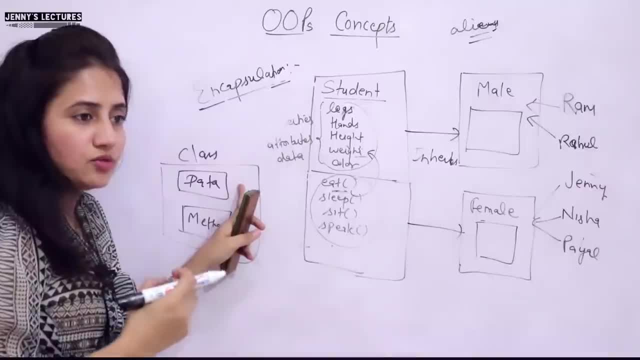 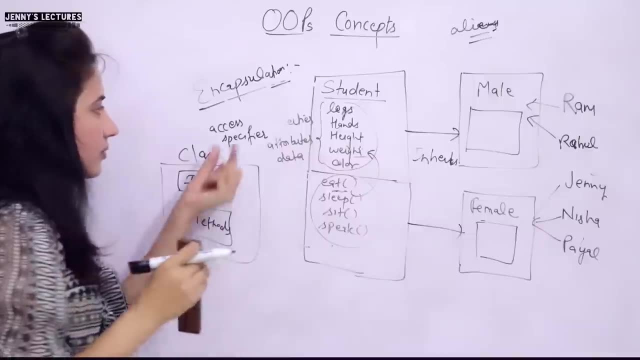 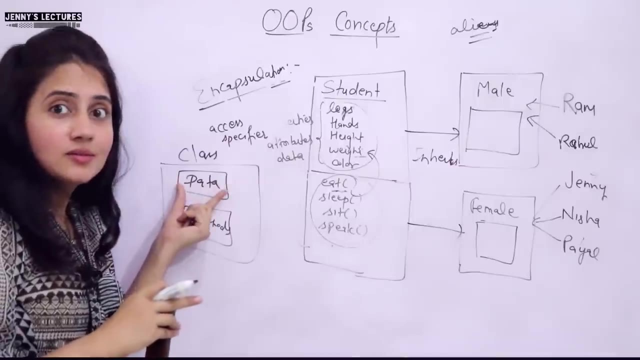 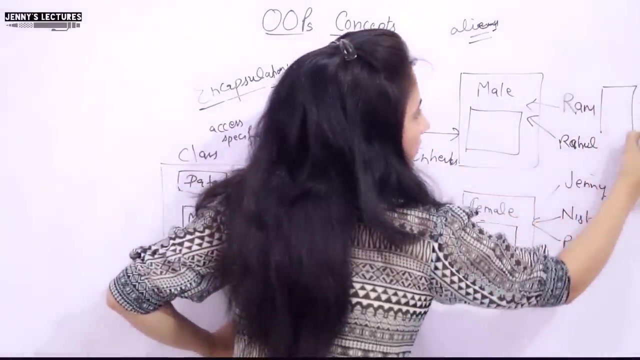 because we have a you know concept, we have something in c++, that's it. so we have data for Ram. you have to add these three methods and this data will generate large sequence on which we can say that r7 is hanging right and this here will be seperated. посмотреть on the data Mulls, because it is highly complex. process as well. right, there are so many different methods there is, so there are two method that are available in c++, so there are different method that are available in pills. there are two methods that are available in dumbelle, which uses r1 to provide kinds of generic Moses. values of x and j. and then third method, which was j, when you want that kind of source, this indeed, and s goes on to let us know in c++ that there will be various methods of r1 that can you connect any originate hardware with this as well? there are so many that you will be able to learn. 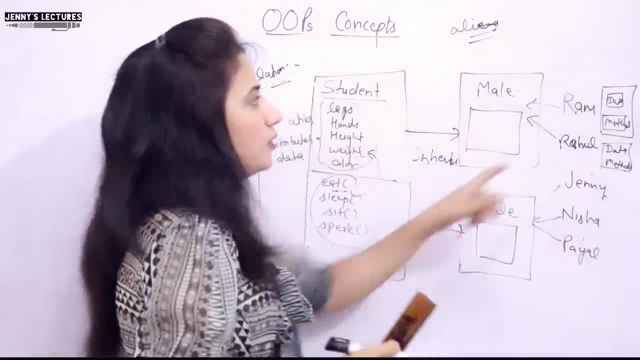 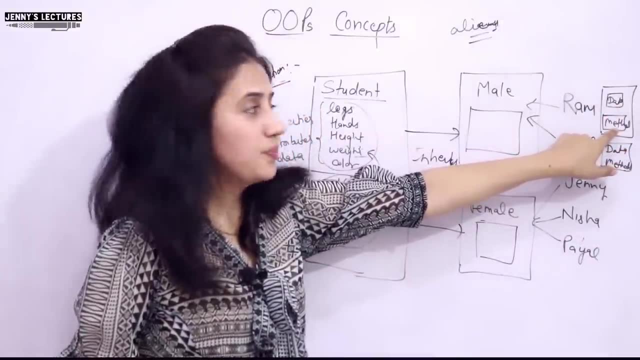 that right which полез building on the display in such a way. now I will keep the data without nehmen. these are methods, So you can keep that data private. Only these functions. these are public methods. So only these functions, these methods can, can what? Access this data, This object? 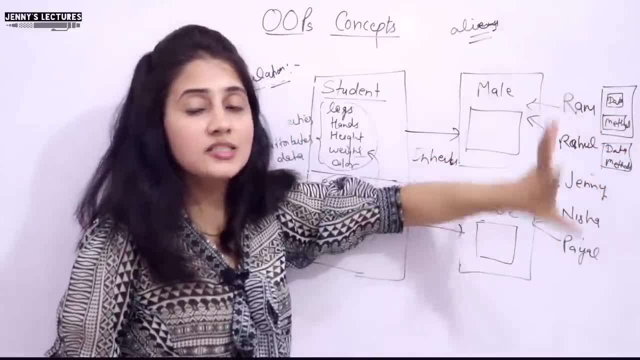 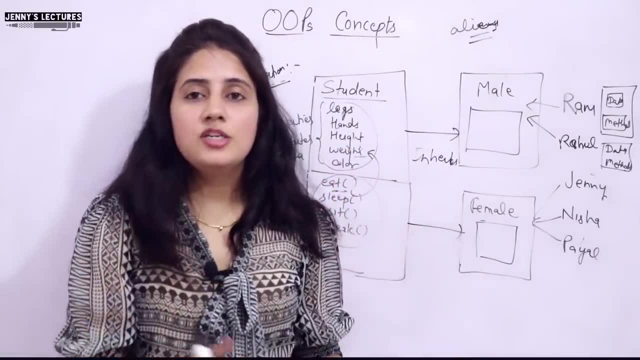 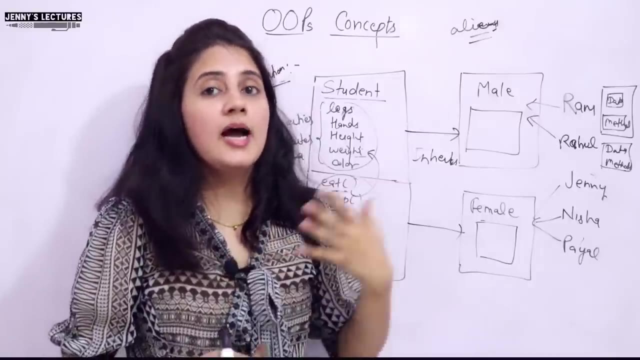 another object cannot access this data or another class cannot access that data. Let's take one example. like we have in college, we have multiple departments- CSC, mechanical, civil, EC, right. Suppose I am faculty in computer science department and I need one. 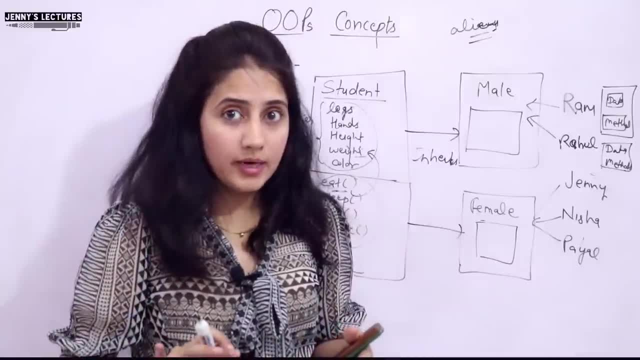 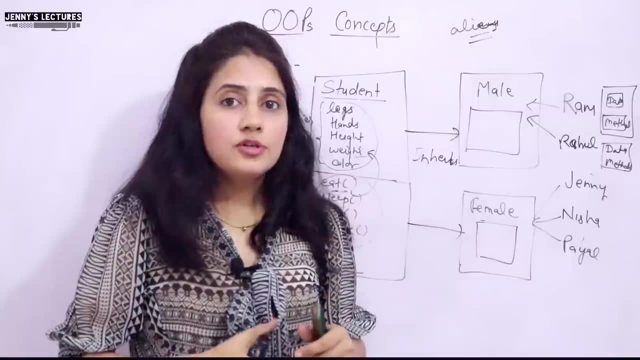 information. I need some data from mechanical department right. So it's not like that I can directly access the data from mechanical department right. I will first talk to. I will reach out to a person in mechanical department right And I I will request to. 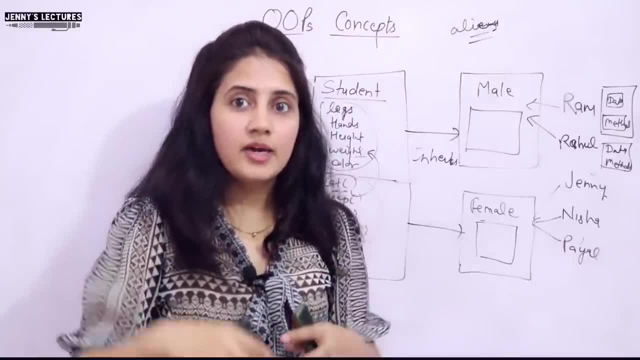 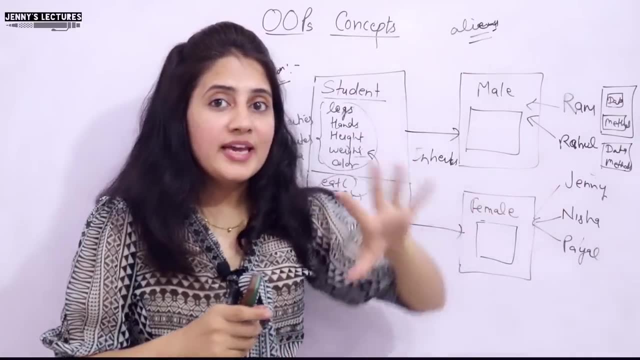 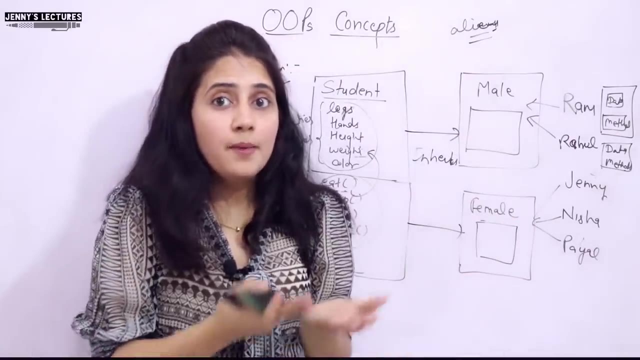 that person to get me that data And after that, through that person, I can access the data right Directly. I cannot access So the data of mechanical department, the employees or the faculties of mechanical department completely. they are a single unit known as mechanical department. 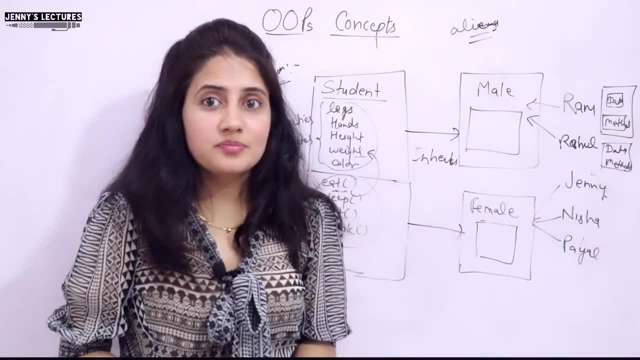 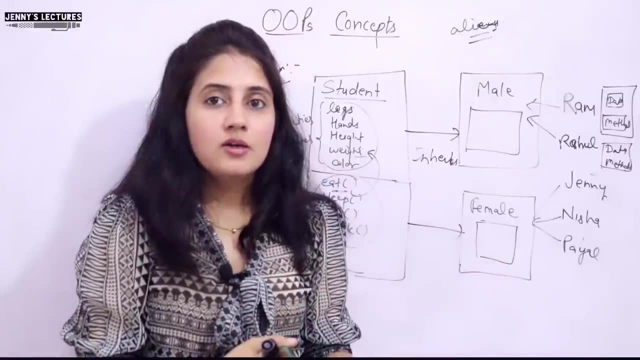 So they are wrapped up, they are encaps- encapsuled So the data is private to mechanical department. only the faculties or employees of that department can access that data. So this will increase the privacy, the security of the data. That is why in the previous video, 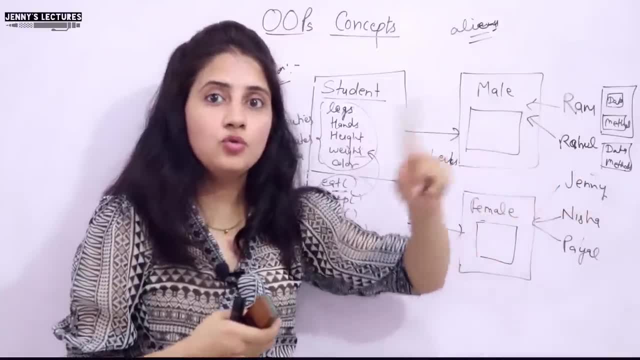 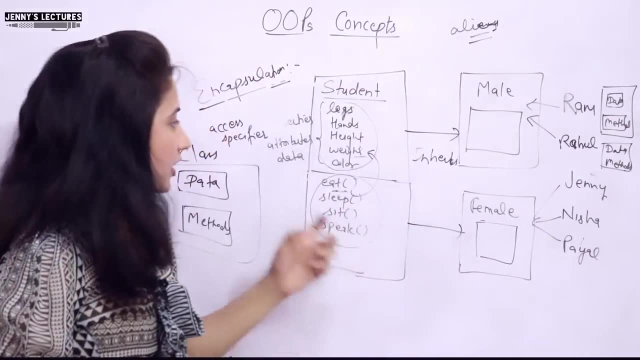 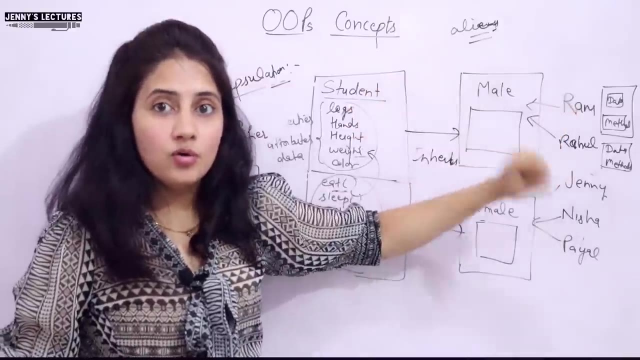 I have told you the main reason we have switched from POP to OOP's: data security, And through encapsulation we can achieve that thing: data security, privacy by keeping the data private, because we have excess specifier concept here. Just keep all your data private And only these methods, only the methods of 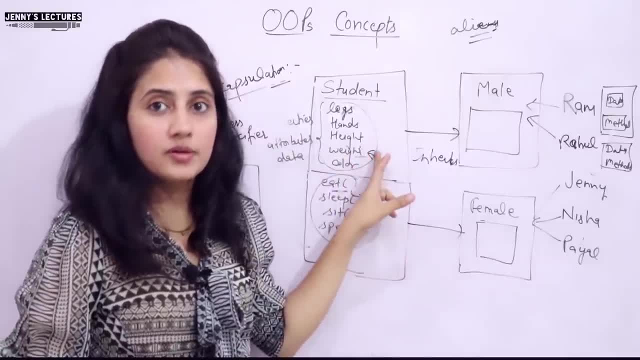 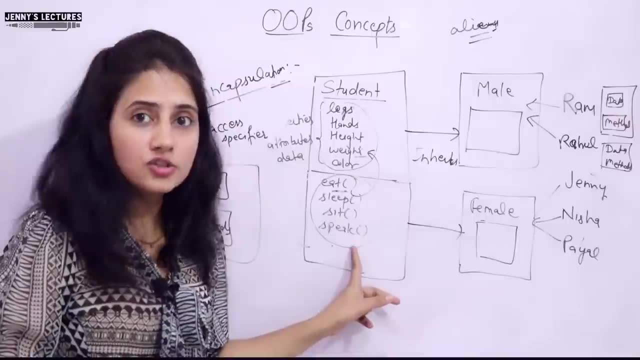 that class access that data, only right. No other class can access that data. If another class want to access that data, they will communicate, they will communicate, they will communicate, they will through these functions right and through these functions they can access that private data. 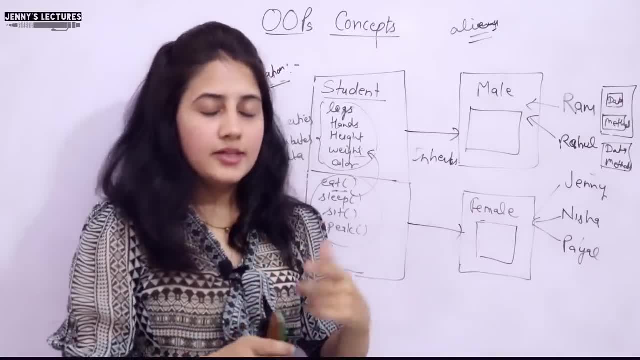 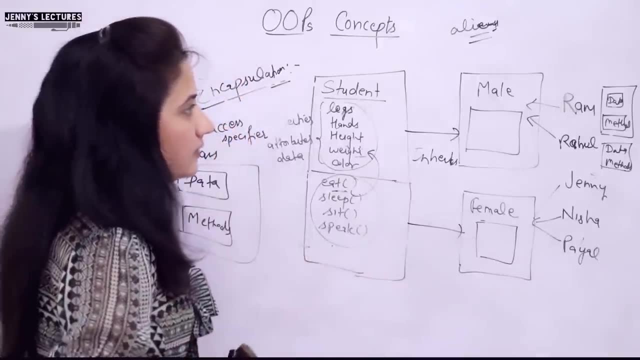 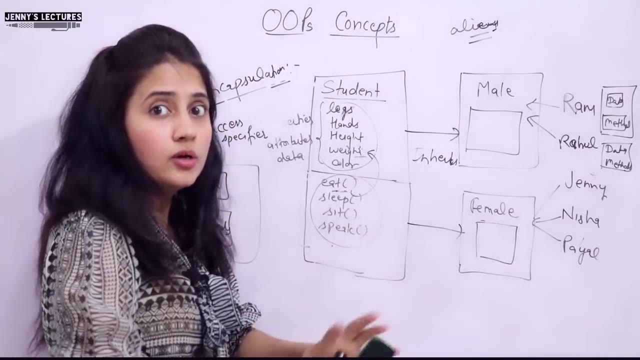 right, We have some concept of friend function, friend class, but that also we will discuss later. we will not go in this much detail. I hope you know the basic idea of encapsulation right? So it is, you can say, just a shield which prevents your data from being accessed by the code. 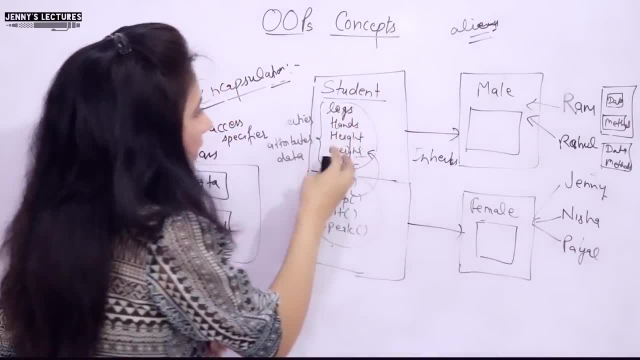 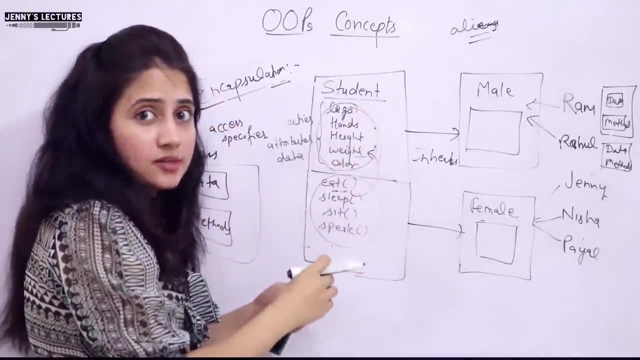 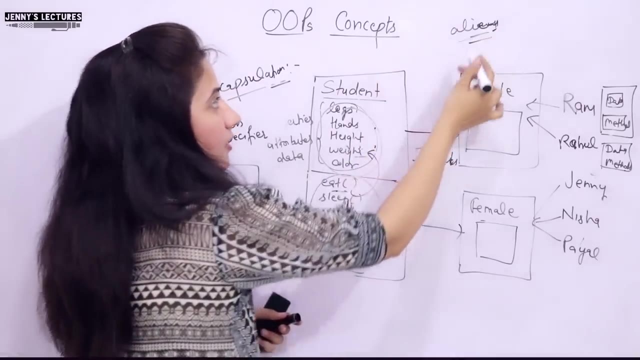 outside of that shield, right, or you can say the data or the variable, this is the data. or you can say the variables of one class can be accessed by the methods of its own class, not by the other class. right, like other class is alien, so they cannot access this data, this data of human being. 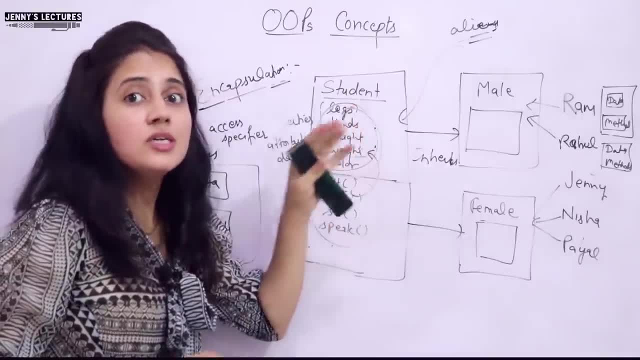 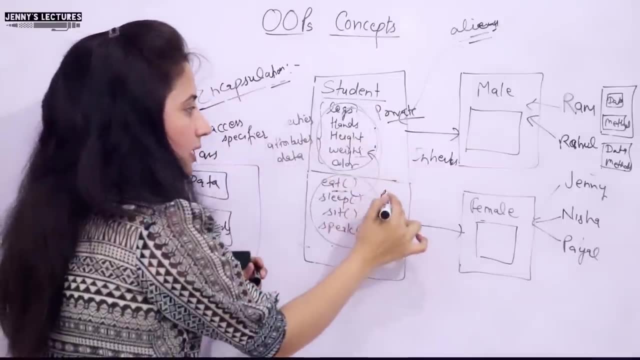 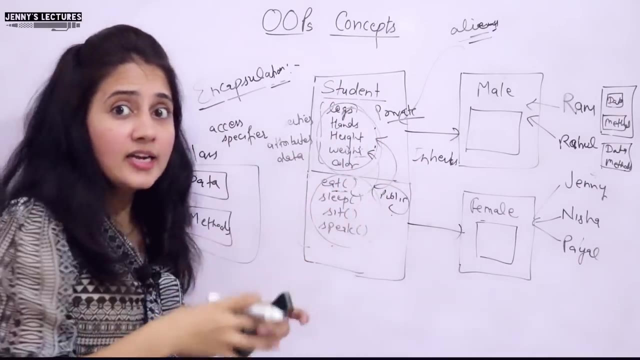 class or a student class, and how to achieve this encapsulation? just keep your data private, use a access specifier private and keep your methods public, and using these methods you can manipulate this data. only These methods, these functions of that class only can access this data- private data. this is how you. 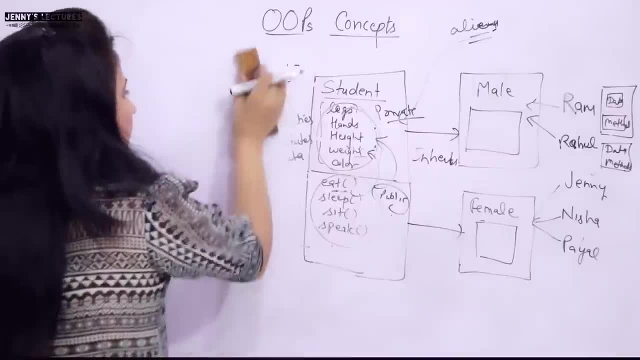 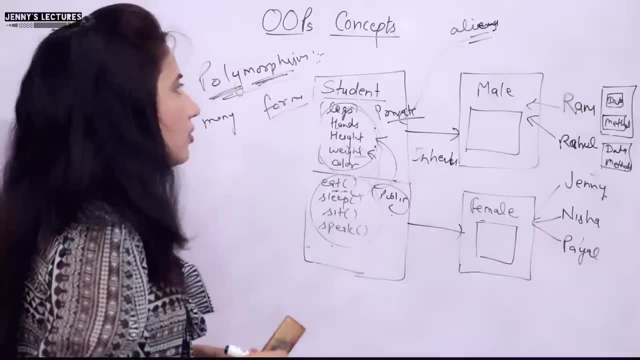 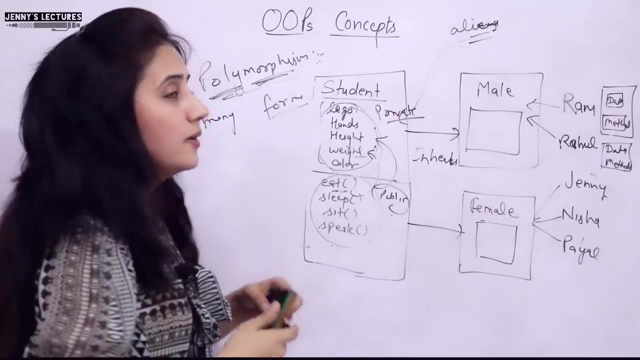 can achieve encapsulation. that's it Now. next is polymorphism. see this: poly means many, and morph means forms, many forms, polymorphism. Now how this would be related. let's take a real life example here. see me: Jenny is one person right, but I have multiple forms. 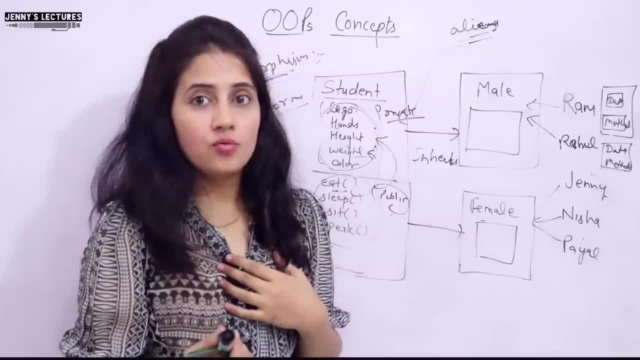 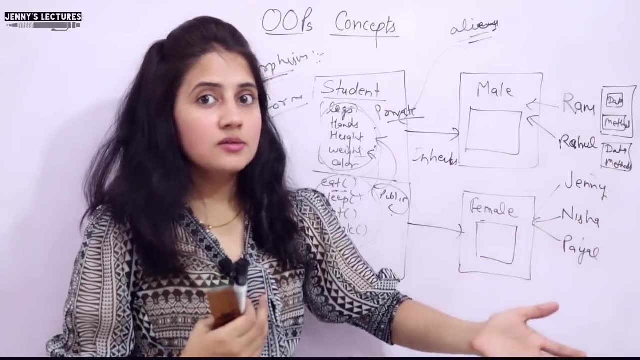 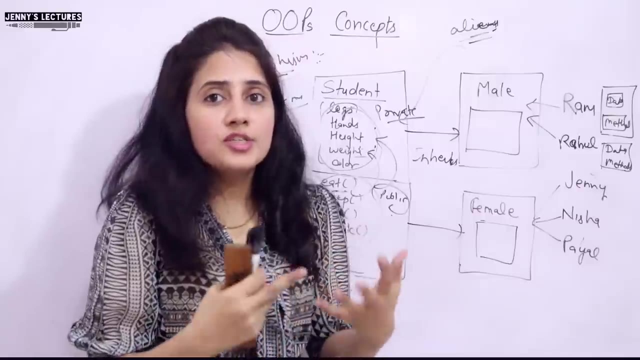 I can say many behaviors or many characteristics I can I have like I am. I am a faculty, right. I am, a suppose, a class teacher, a tutor of any class, or a friend or a colleague, so with according to the situation, I will change my behavior. Jenny is one, only, one person only, but having multiple forms. 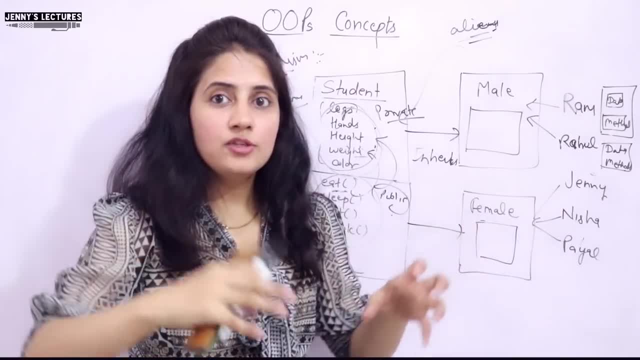 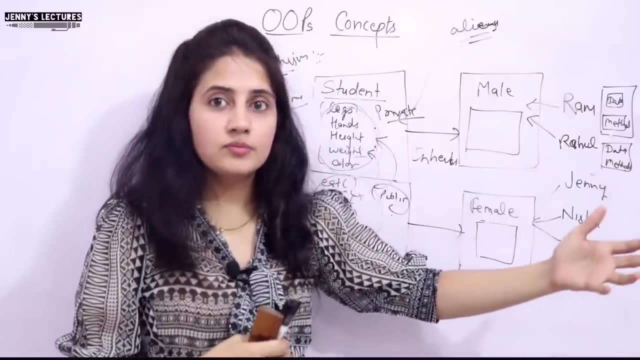 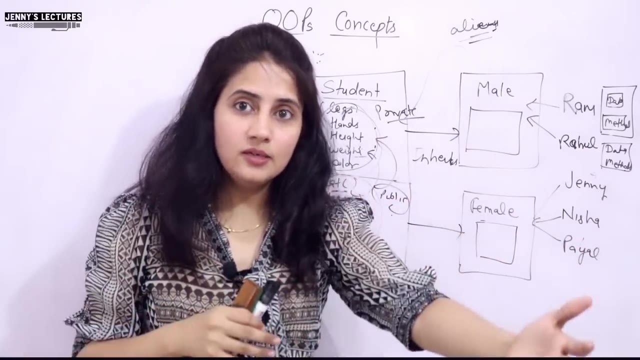 as a faculty, like if I am interacting with HOD, my behavior would be another. It means different. if I am in class as a class teacher or a tutor, then my behavior would be different With a friend. my behavior would be different with my colleagues, suppose not friend, but just a colleague. 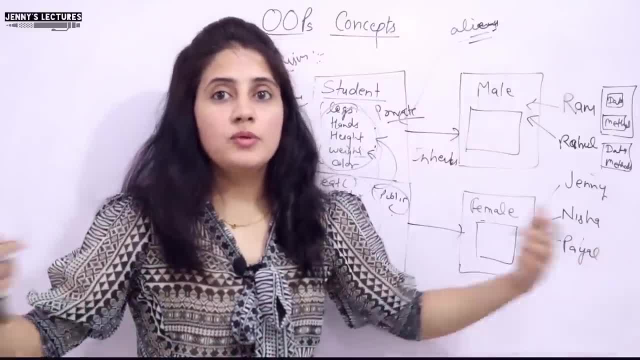 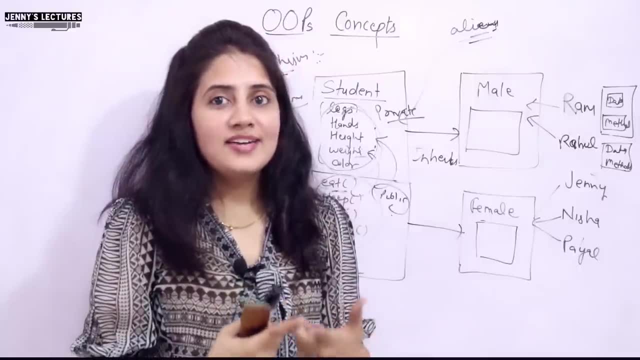 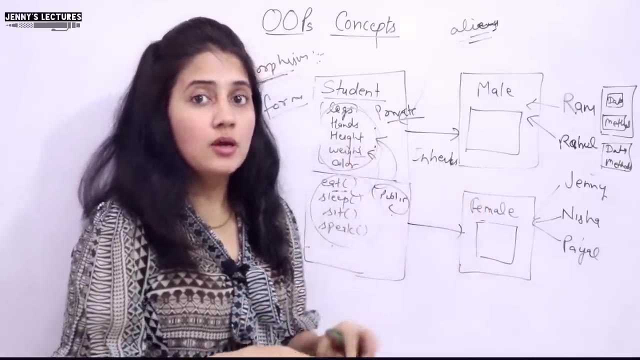 my behavior would be different. right, so I can have multiple forms, but person is one. so this is what polymorphism right now, how you can relate this in programming. in programming, we can have two types of polymorphism, or we can achieve polymorphism by two types. 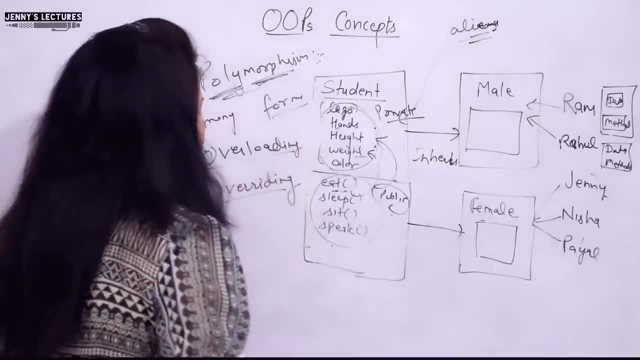 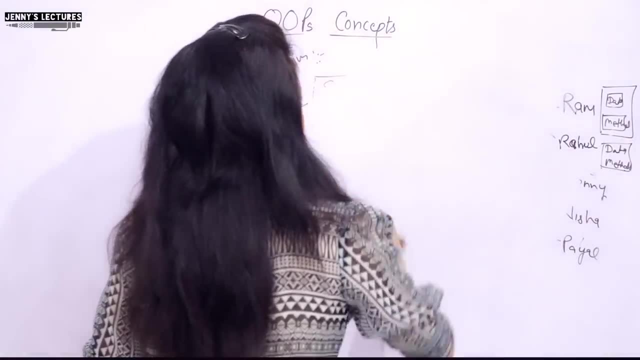 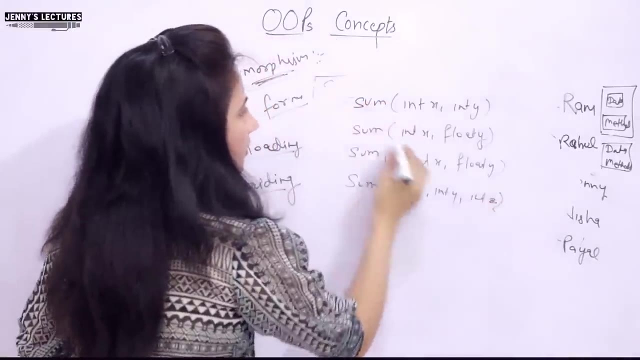 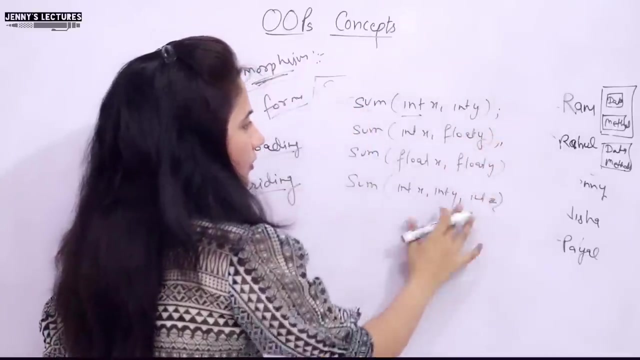 One type is overloading and overriding. see what overloading means. let's take this example. we have a function. let me just rub this first. suppose we have a function. some suppose we have this function. some one function is this: I haven't written properly, right? some read: I want to be there, semicolon and all we have. but it just just to get you familiar with this thing. 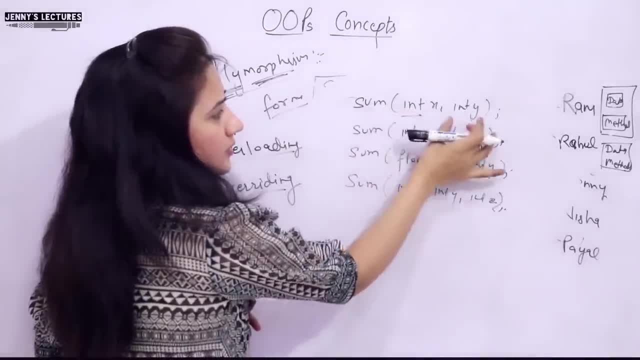 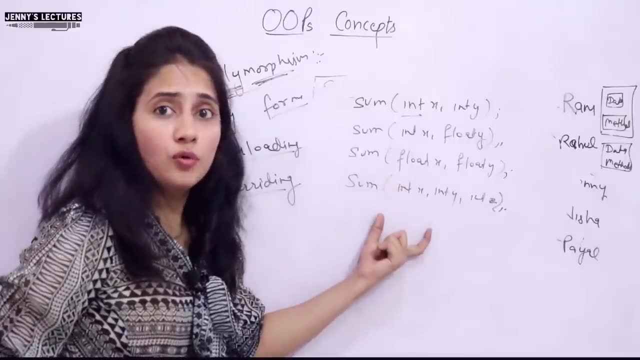 This function is having two arguments, So it is a function. It is a function integer. This function is having one int, one float, two float. This is having three arguments, right? So this is what overloading of the function. The function name is same, but it will do sum of. 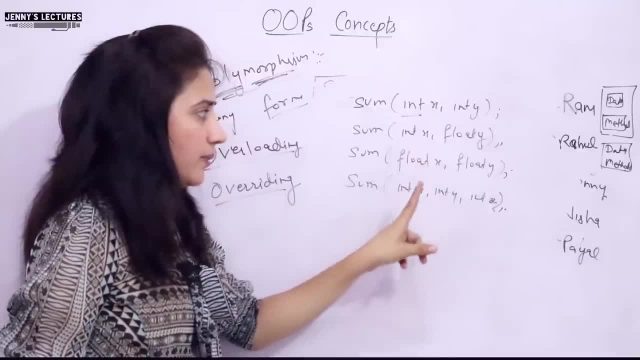 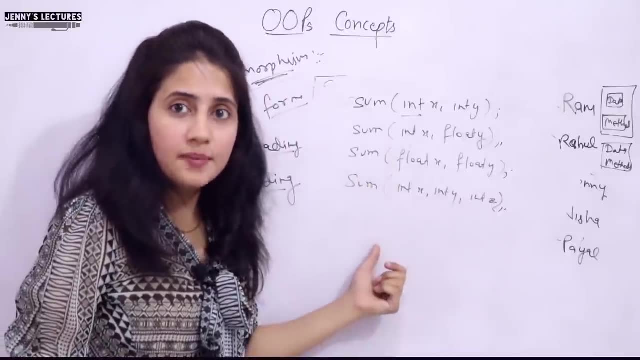 two integer, It will do sum of one int, one float. It will do sum of two float number. It will do sum of three integer numbers. This is what overloading, Just function name would be same. Maybe you can change number of parameter, the type of parameter, the return type of that function, According to. 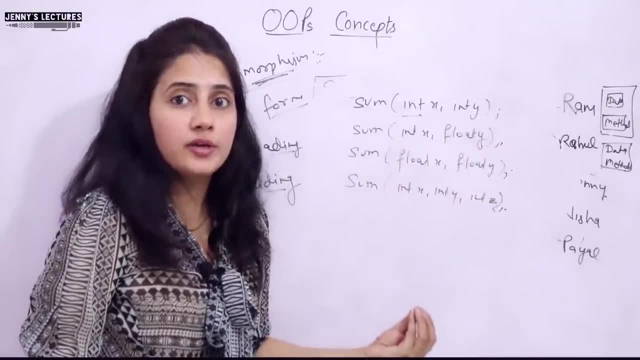 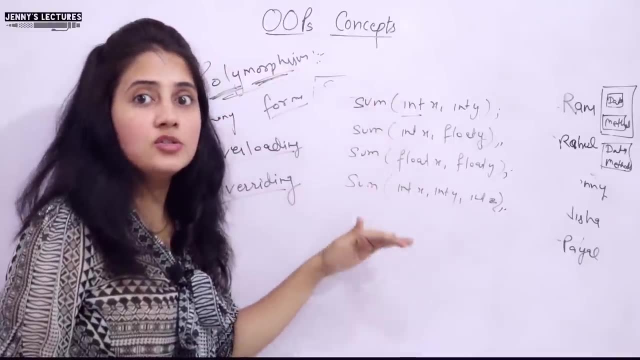 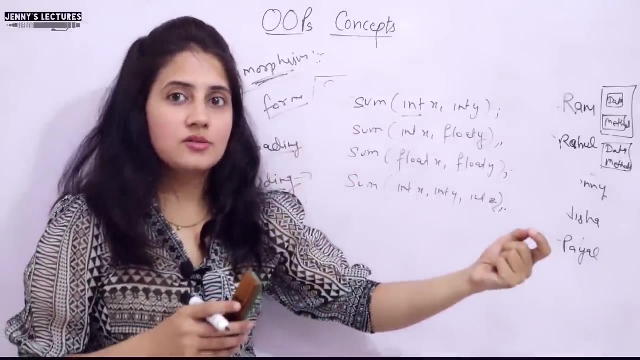 that that function will behave differently. So this is what overloading of the function sum. So this is overloading. Function is same but having multiple forms, One is overriding. Overriding means what Actually? overriding allows a child class to override a function which is already. 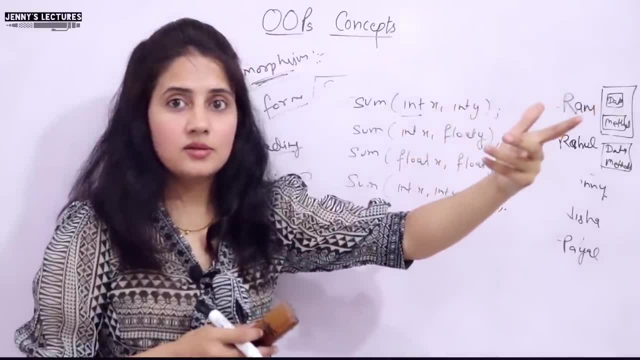 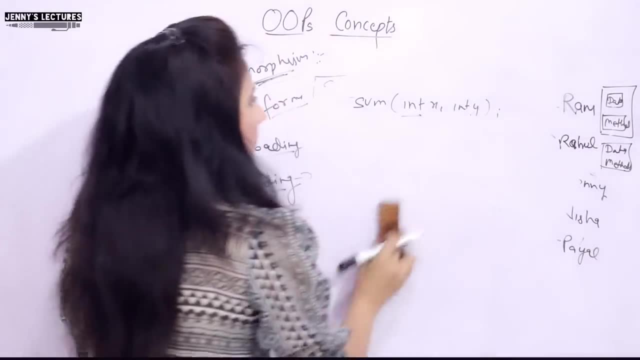 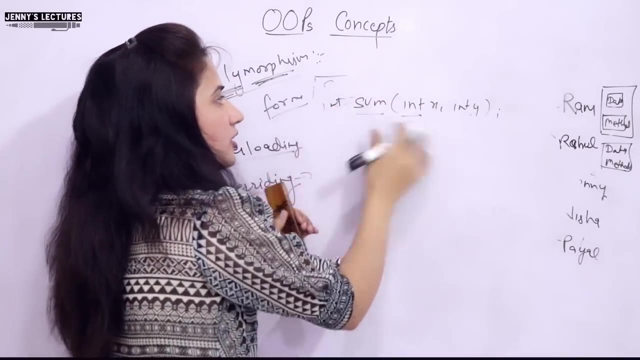 defined in its parent class, right Like. let us take this example: This is overloading And in overriding function name would function would be same Function name, number of argument, type of argument, the return type of the function, everything would be same, Just we change this. 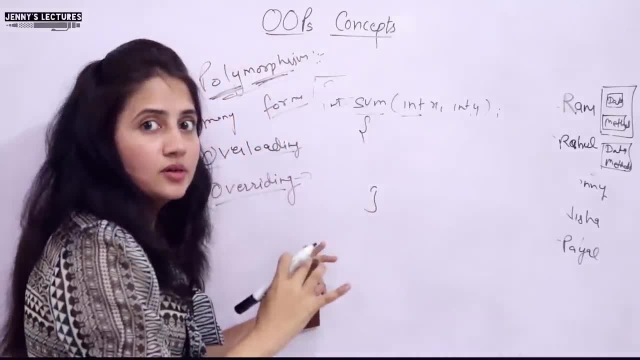 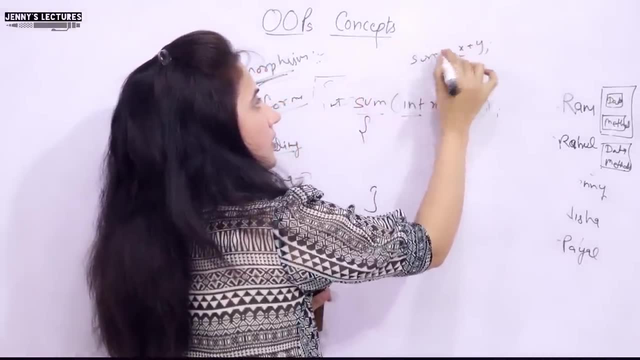 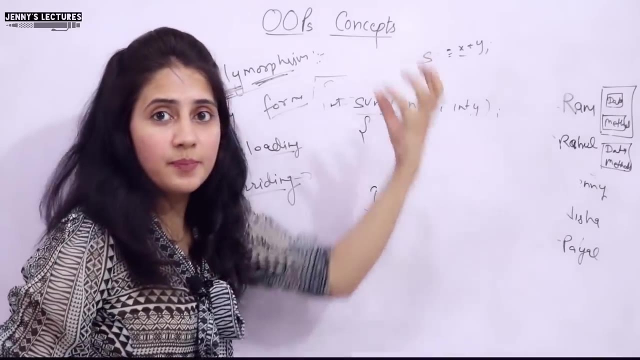 code, the implementation thing, the mechanism. Suppose in parent class sum is equal to a x plus y. This we have done. A sum is a variable. or you can say: another variable is what S x plus y Maybe will inherit this thing from the parent class but totally change the implementation and it will lose. 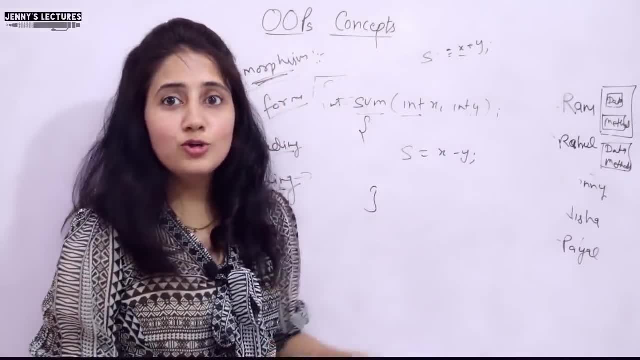 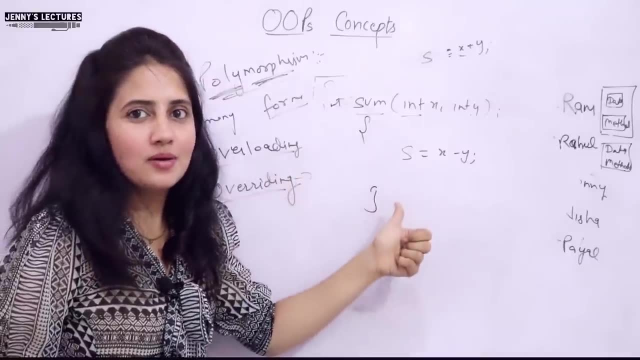 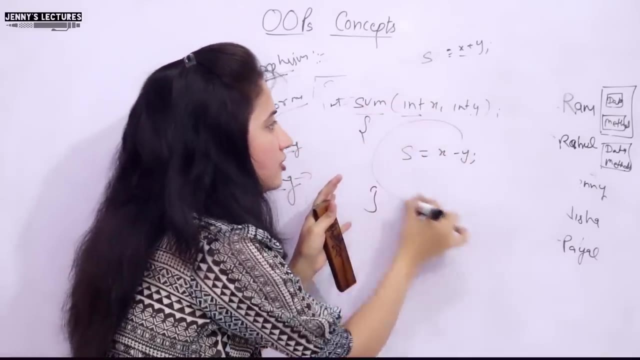 sum is equal to x minus y, Although it's not correct, but I just want to, you know, differentiate the overloading and overriding with the same example, right? So I have just everything is same: name, number of argument, type of argument, the return type, everything is same, but we have changed. 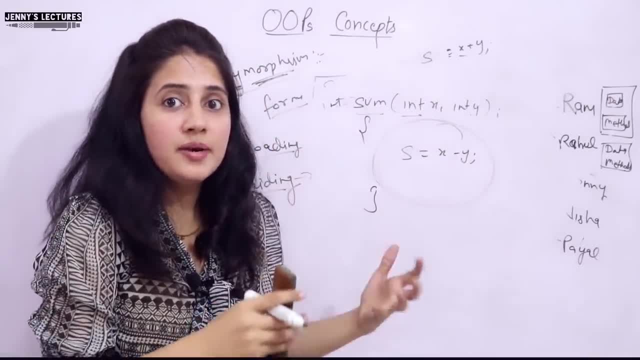 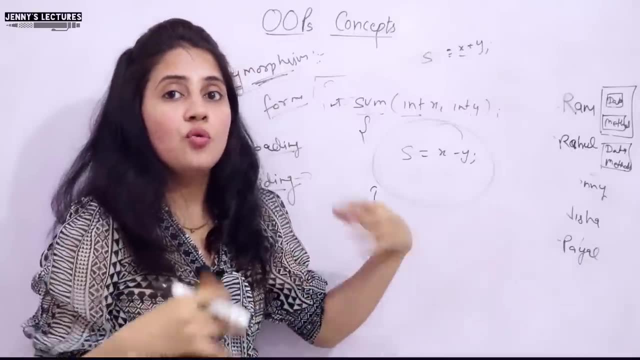 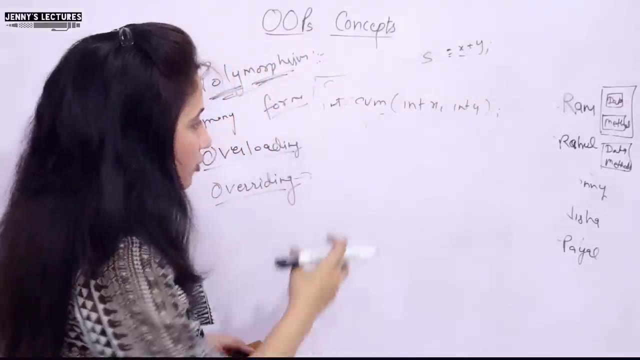 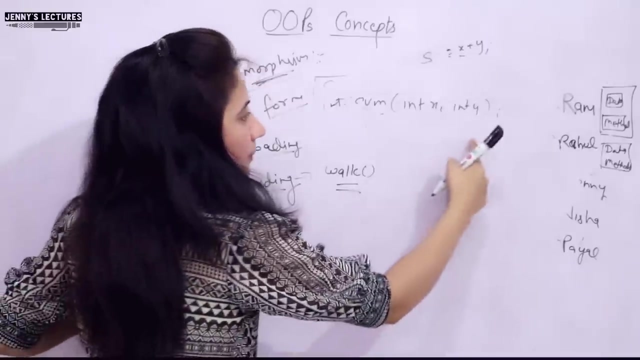 the implementation detail. The child class has implemented that function specifically according to its need. So this is what overriding of that function right? Let's take that example, real life example. Suppose here we are, we were having a function, what work right and male and female will. 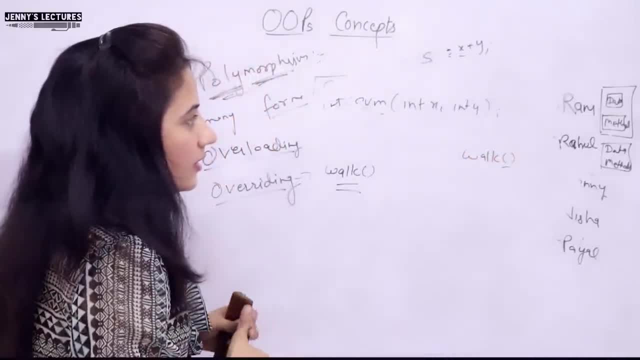 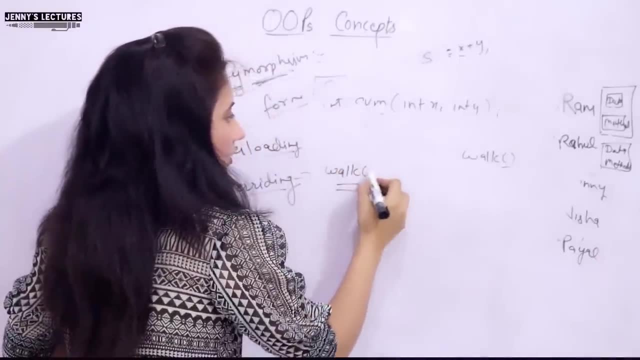 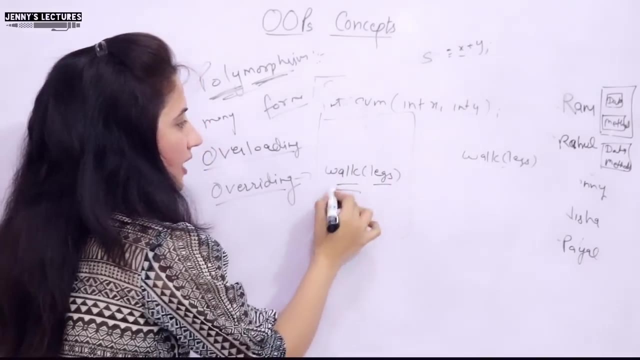 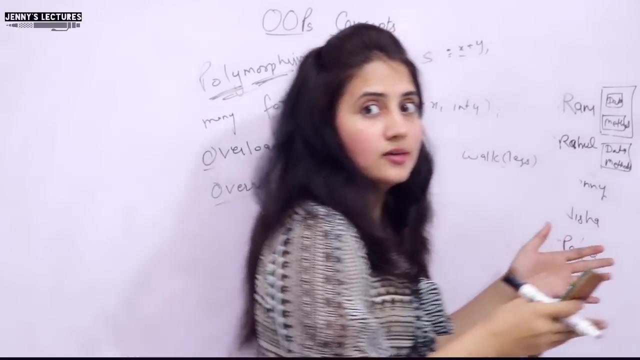 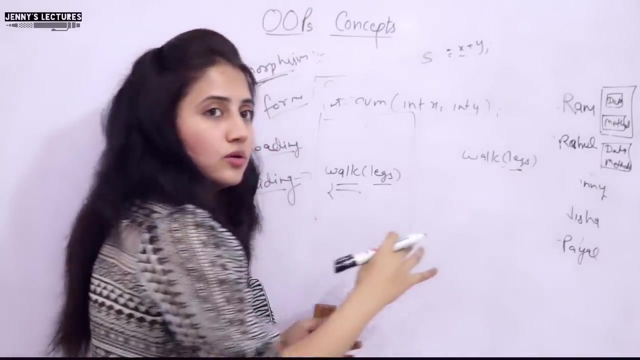 inherit this function work right. So male and female according to their self. they can modify this like walk with legs. argument will pass legs. but in student class, in parent class, it is what? normal walking like this we can walk right, fine, it's normal walking and they override this function. walk with legs: the same thing, but 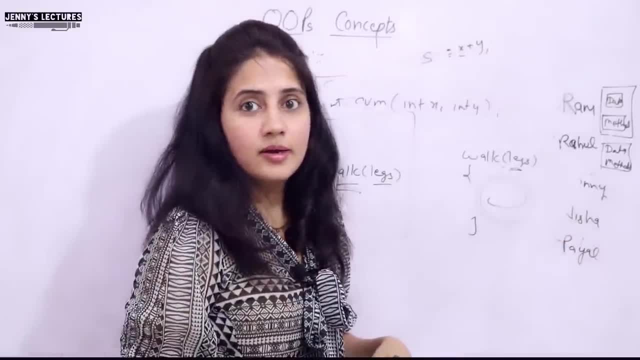 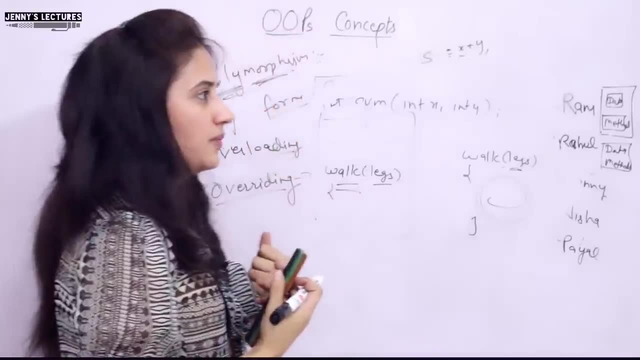 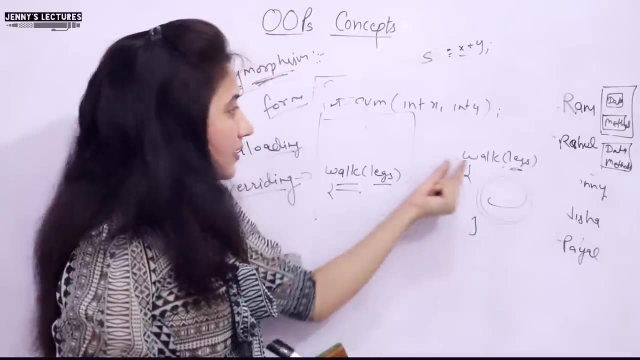 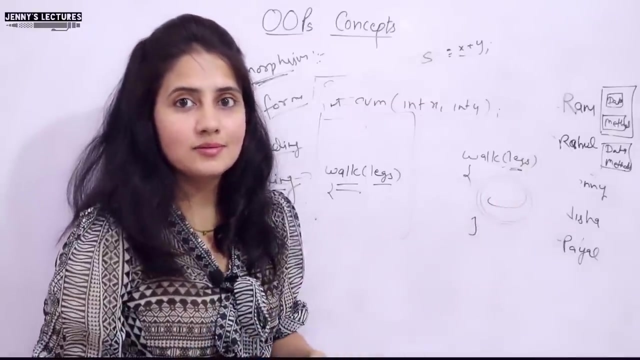 they change this part, this implementation part- Suppose female class, they, they will change this part, walk, reverse, something like this. So they have changed the mechanism of walking. although the name is same, argument is same: they are walking with legs, but they have changed the mechanism. So that is overriding right and overloading means what simple if you take this.